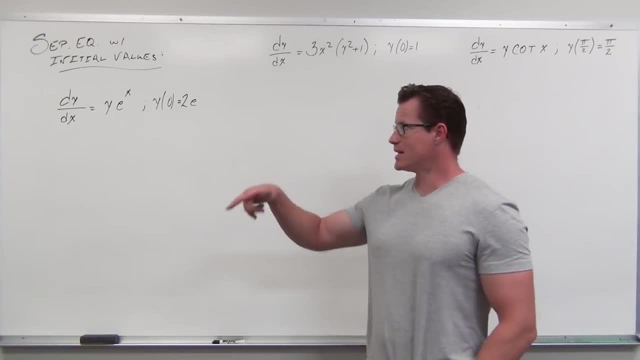 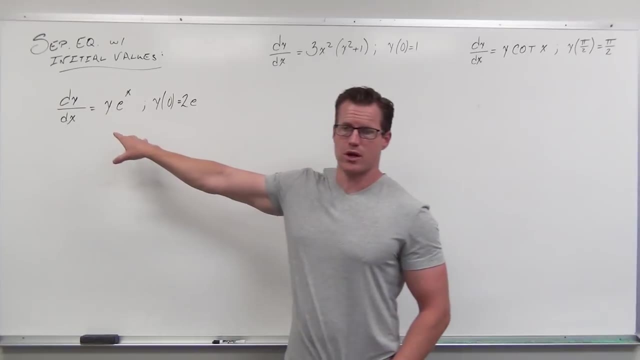 So we've got a differential equation that's equal to dy. dx equals y times e to the x. So we're noticing first, right off the bat, that we have derivative equal to product with x's and y's. That's exactly what we're looking for for. 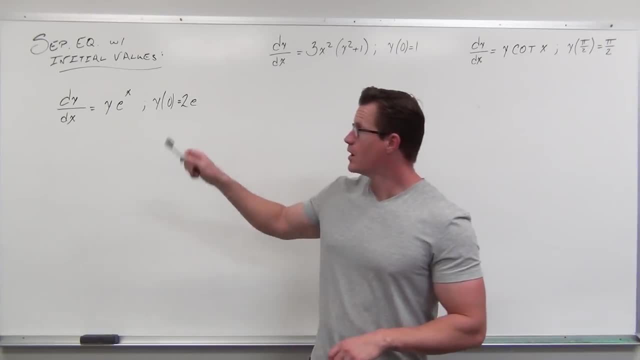 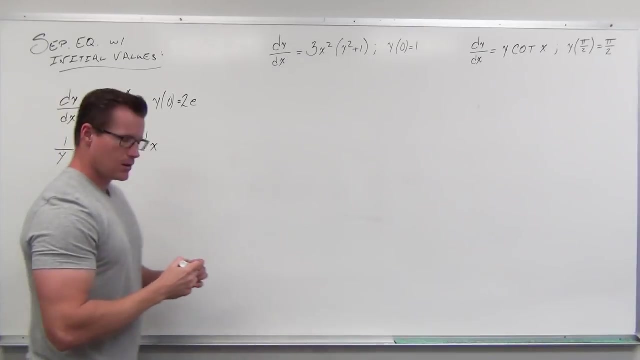 separation, separable equations, so these separation variables. So we're going to do that. We want to group our y and dy on one side, x and dx on the other. So we're going to do that, Just like that. Maybe divide by y, leave the e to the x and move our dx over. 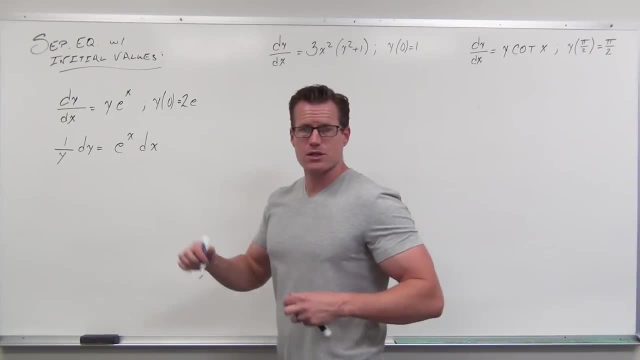 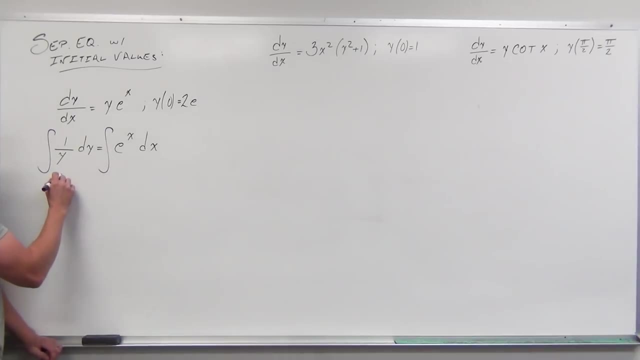 Now we can take an integral and we know that integrals undo derivatives. so if we integrate both sides, on the left-hand side we get this a lot, this ln absolute value of y On the right-hand side, in the easiest integral or derivative ever. 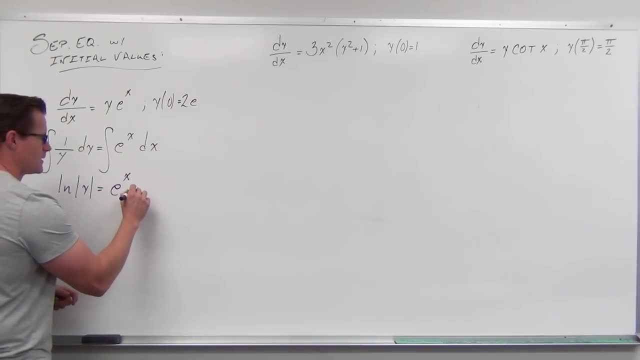 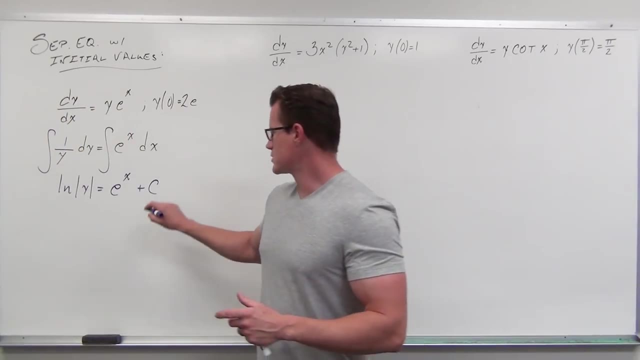 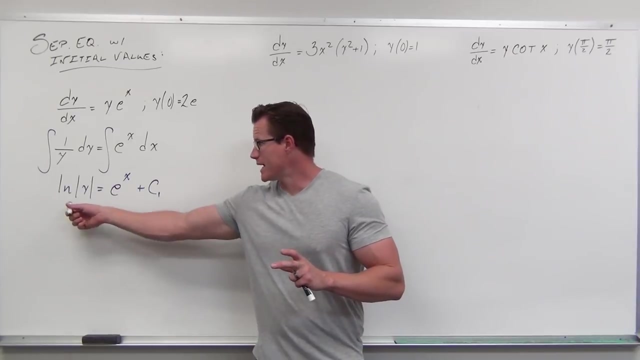 thank you. we just get e to the x, But we also get an arbitrary constant. I often will call this c sub 1, because we can change that. Now, here's something you need to know: Even if we change that c sub 1, because we're about to get an exponential on this- even if you get that to be like 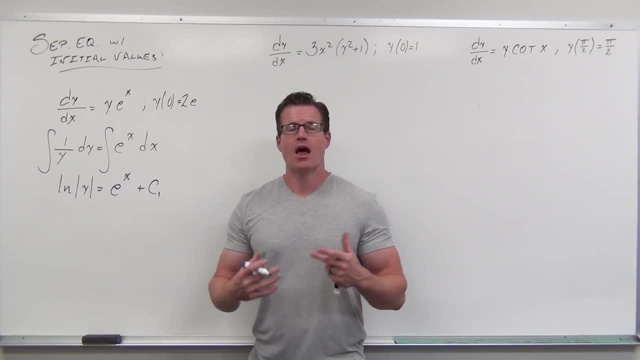 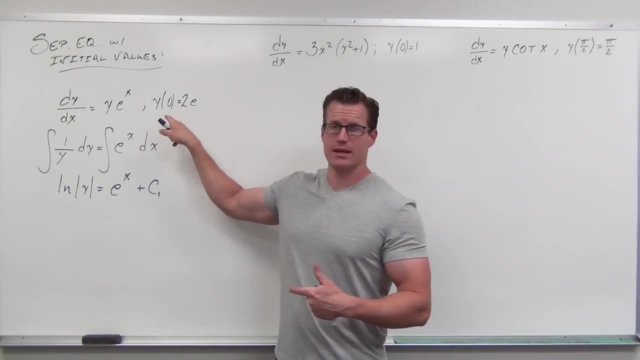 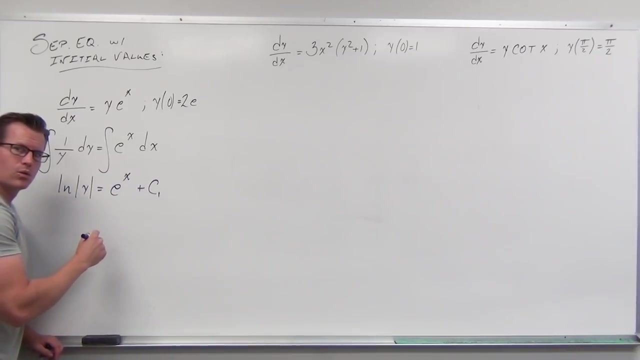 plus or minus e to the c sub 1 and you call it c. that's okay. So sometimes it's beneficial for us to do all of that work and then plug in that initial value. Let me show you that right now. So if we have ln, absolute value, y equals all this garbage. we know that in order to get rid of a natural log. 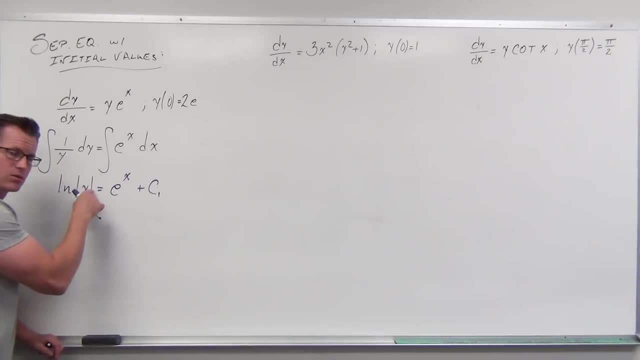 we need a base of e. So e to this side will equal A value y. That would be e to the e to the x plus c 1. That looks really awkward, So let's fix just a little bit of it. Let's take this: We know that if 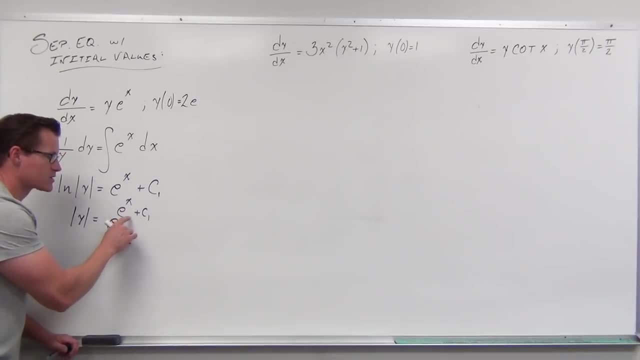 exponents are multiplied. they came from- sorry if exponents are added- they came from bases that are multiplied. So absolute value of y equals e to the c, sub 1 times e to the, e to the x. Common bases being multiplied gives us exponents that are being added. I just 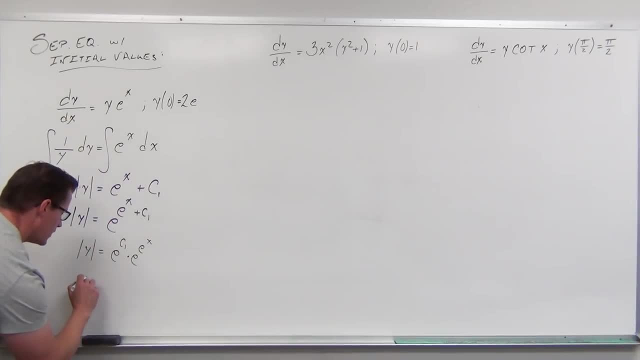 switched the order. Also, we know about absolute value. y would equal plus or minus e to the c, sub 1 times e to the e to the x. Now I want to show you that this is possible. This is why we didn't plug this in earlier. We. 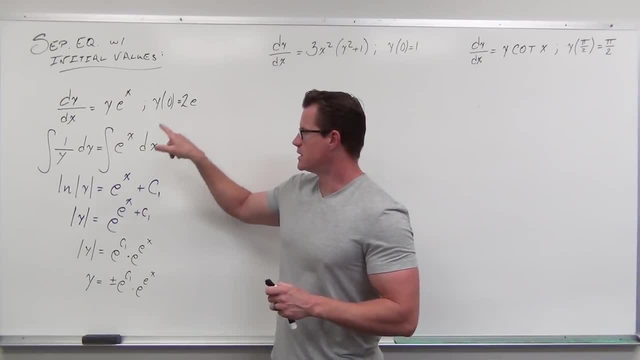 could have taken this initial value, plugged it right there and solved for c. That would have been fine. We would have had 0 for our x, giving us 1.. We would have had 2e for our ln- giving us- probably not here, but giving us ln of 2e- and we could separate that We'd get ln of 2,. 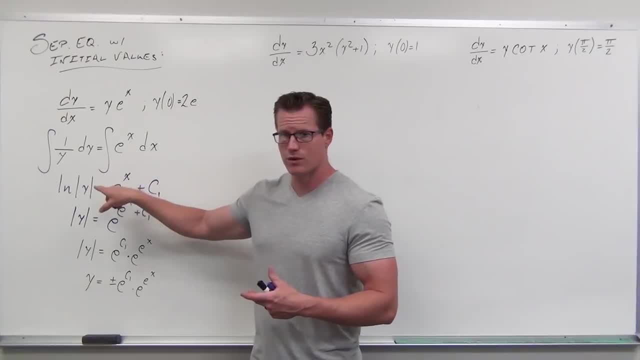 2e Plus ln of e, which would give us 1.. Subtract 1 from both sides, c would equal ln of 2.. You could totally have done that, And then this would be ln 2. That would be ln 2. We'd get e to the ln 2.. 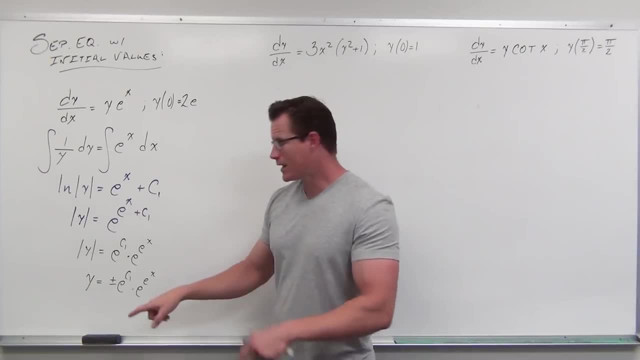 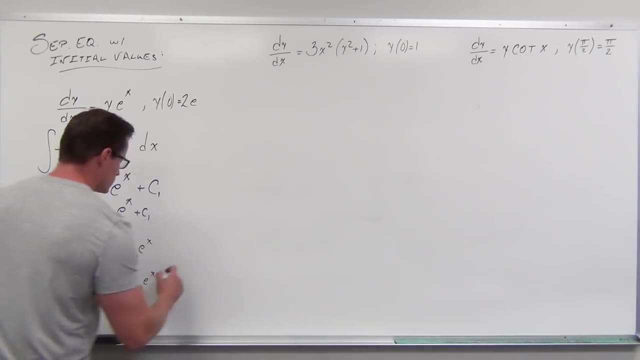 Oh, my gosh e to the ln 2 is 2.. So what we're going to find out later is that this is going to be 2.. You can do exactly the same thing later on. So if we call all of this just c, let's just call. 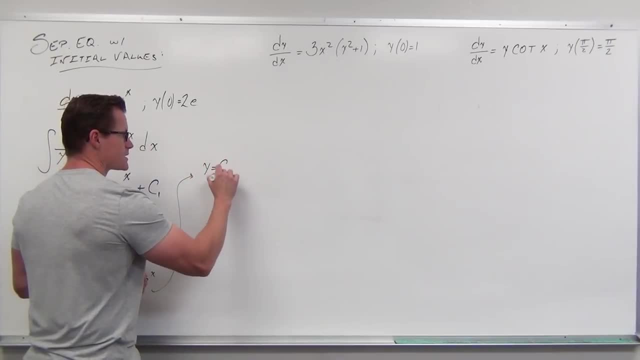 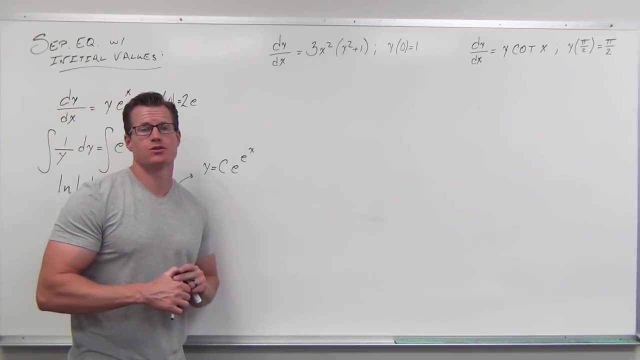 that big c- We've done that many times- Then why? c equals c, e to the e to the x. Once you've got there, we need to get rid of that c, And so how we go about doing that is by using our initial value. We're saying: this is a family of curves. 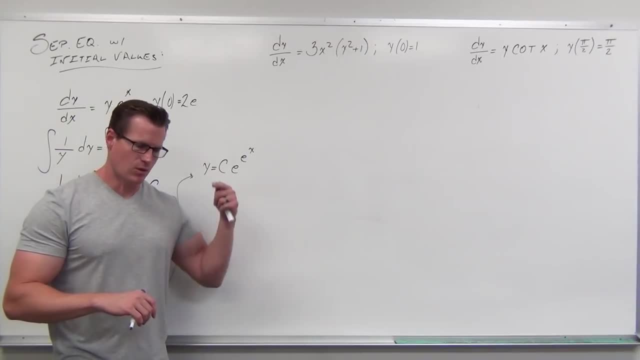 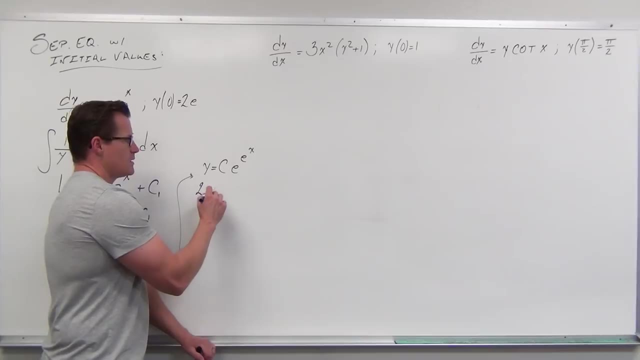 an infinite family of curves that don't intersect. That means that only one of them is going to go through that point. So let's find the c that makes that happen. y is 2e When x is 0. So e to the 0 is 1, which means that we have 2e equals c times e. Let's divide both. 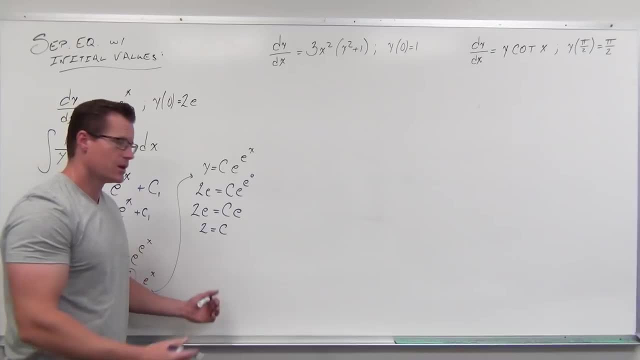 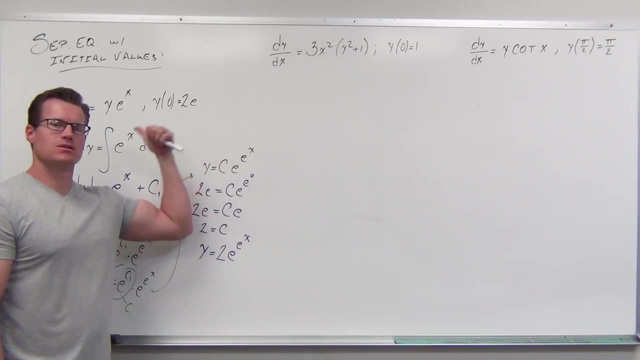 sides by e, c is 2.. So y equals 2e to the e, to the x. That right, there is no longer a general solution, That's a particular solution, The one equation, the one solution that goes through that point and still satisfies that differential equation. 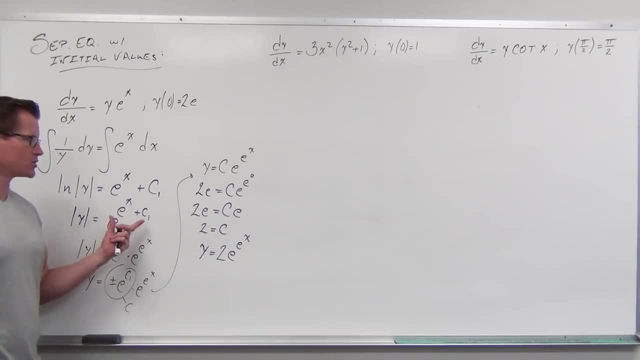 That's what we're looking for Now. I mentioned to you before, I said it in words. but what if you had gone ahead and plugged in this even here? I don't know if I would do that. I'd probably wait. 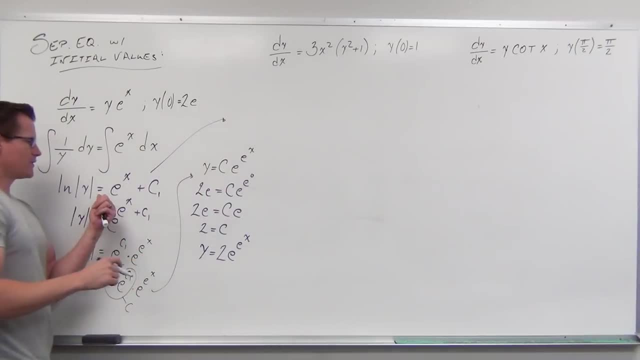 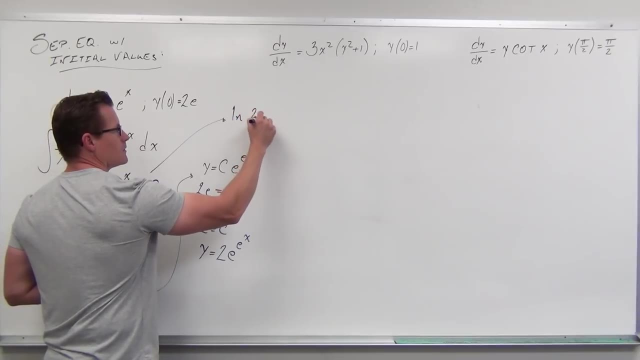 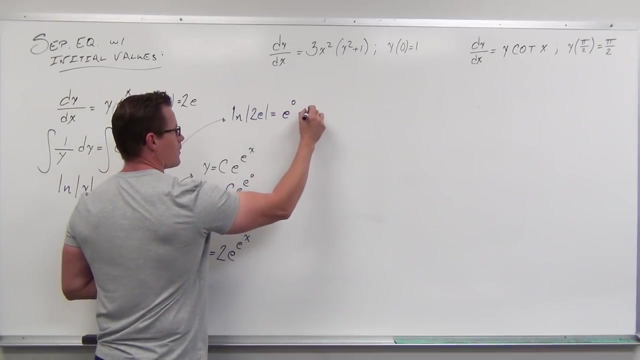 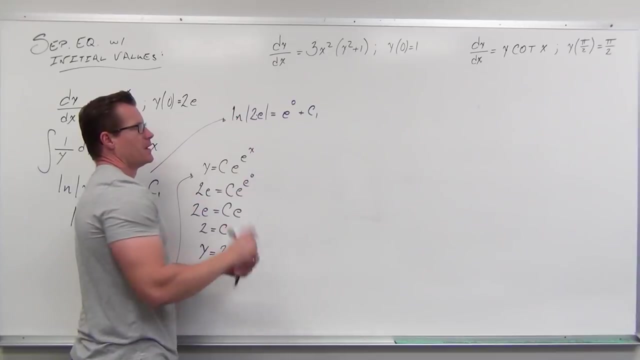 till here, but it doesn't matter Watch. So if I plug in 2e for y and 0 for x, well, this right here is a product. Now 2e is positive, so we can drop the absolute value. 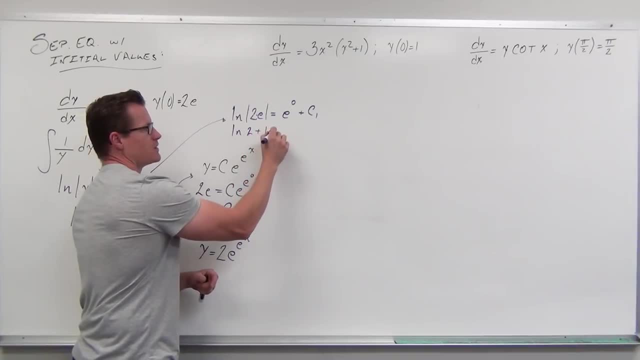 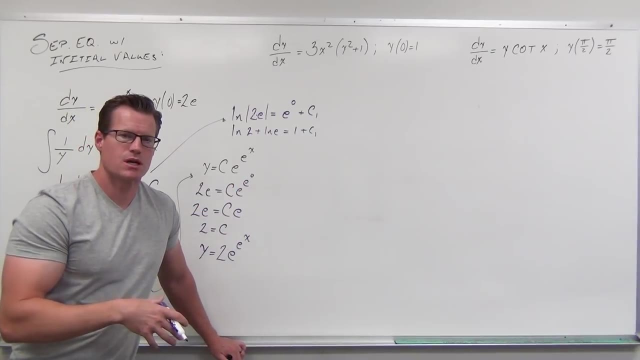 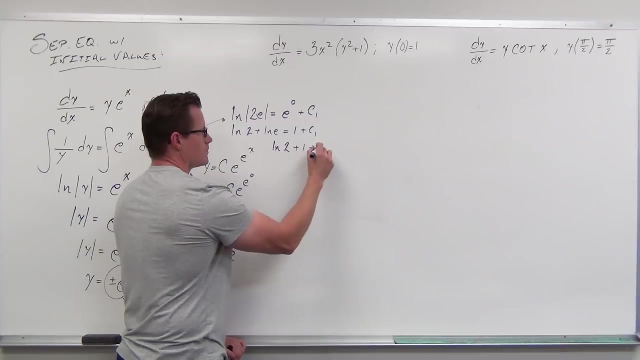 but a product in logarithms can be split up by addition ln of e. you've just composed two inverse functions, So what that's going to give you is just 1.. 1s are gone if you subtract 1 from both sides and c1 would equal 1.. 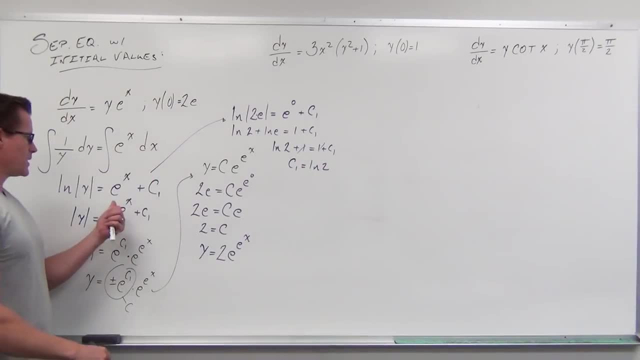 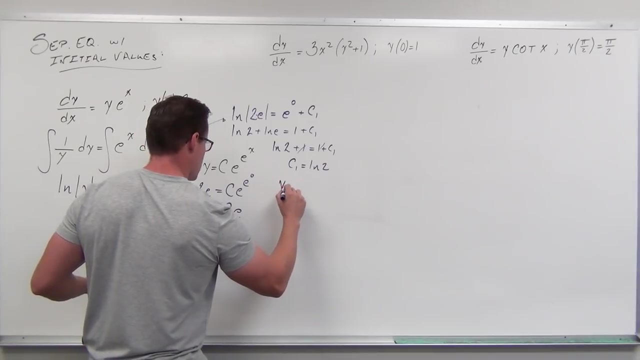 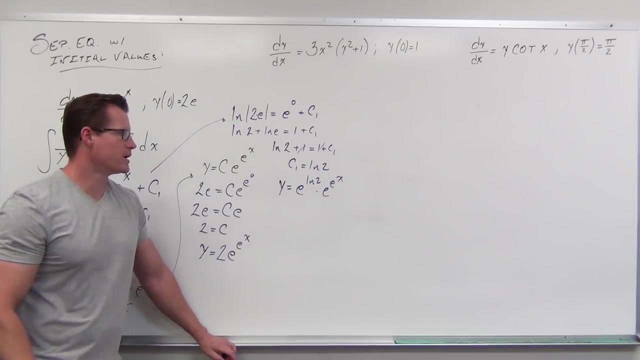 So what happens here? if we have this, let's move all the way down to. Let's move down to here. If we know that c sub 1 is ln of 2, it's all positive. we don't need to worry about the absolute value anymore. 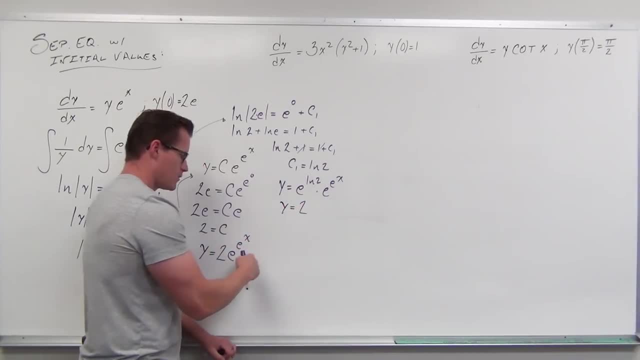 But e to the ln of 1 equals 2 is. I don't know if we actually even prepared this. as far as e to the y, We're just about out of there, But e to and 2 would give us the same exact thing we found here. The question is, which way is? 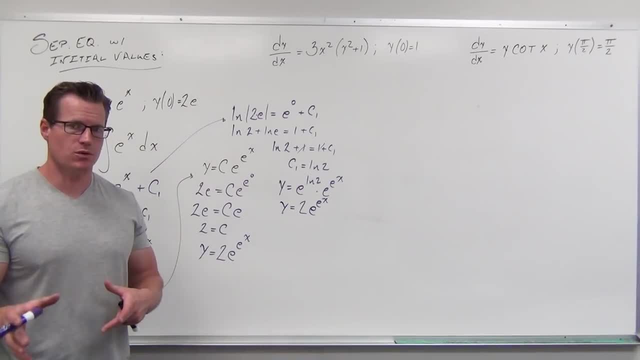 easier. That's subjective. Which way is easier for you? For me personally, I like wrapping all of this up as a gigantic C and then plug it in my initial value. You can do that lots of times. Sometimes it is beneficial to plug it in earlier, so 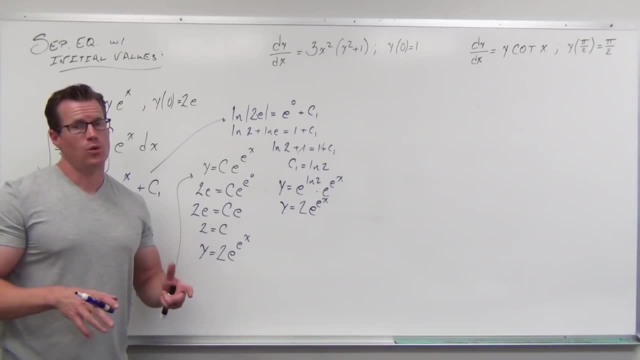 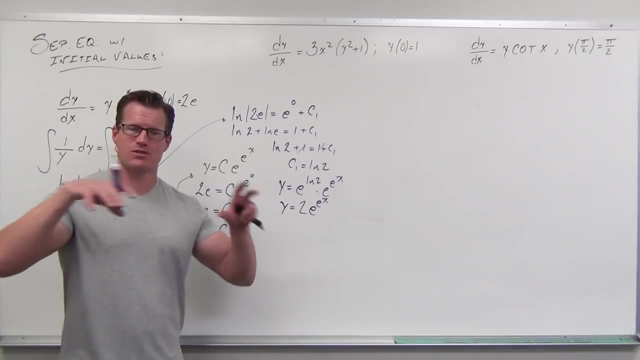 that's really up to you. Does it really matter? No, but for some problems one way is a little bit easier, So keep that in mind as you're going through this. The idea is still the same: separate your variables, integrate, but now at some, 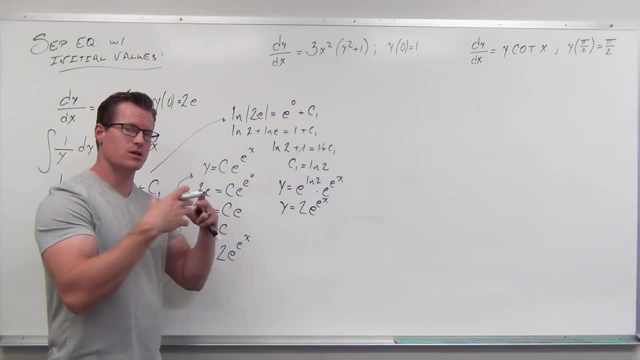 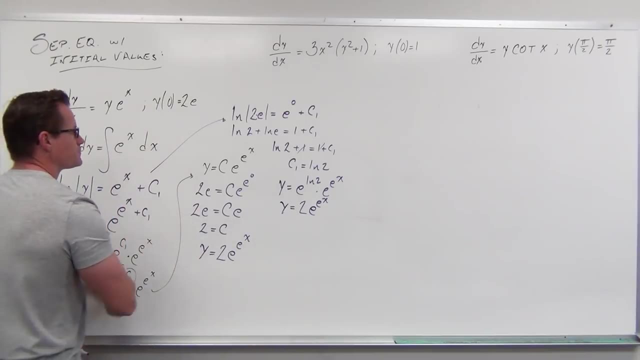 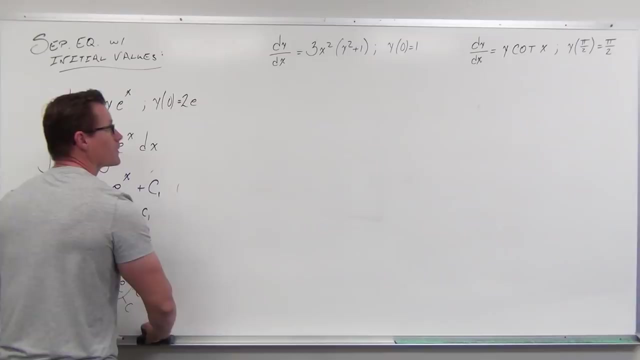 point. we're plugging in our initial value And we're going from our general solution to a specific particular solution using that initial value. Let's try a couple more. So next up, the first thing we're looking for: we have a differential equation. We 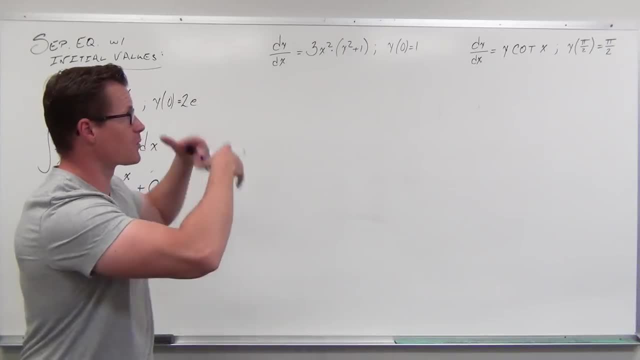 see a big product in there: Group our y is dy, Group our x is y, which makes an expression 4 or 7. You can take and split that with your x is dx, so 1 over y squared plus 1 dy looks good. 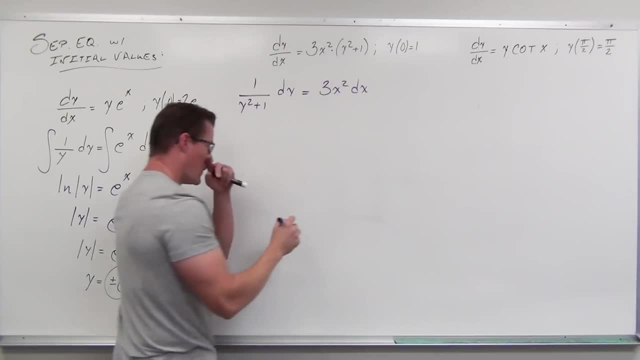 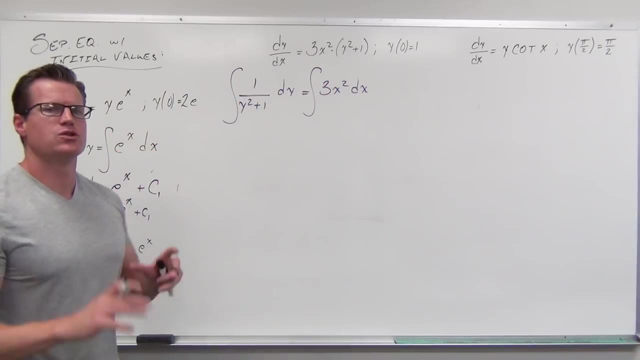 On the right-hand side: 3x squared dx. that's fine. We know that we're going to integrate as soon as that happens. so y is grouped with dy, x is grouped with dx. On the left-hand side. use your tables. 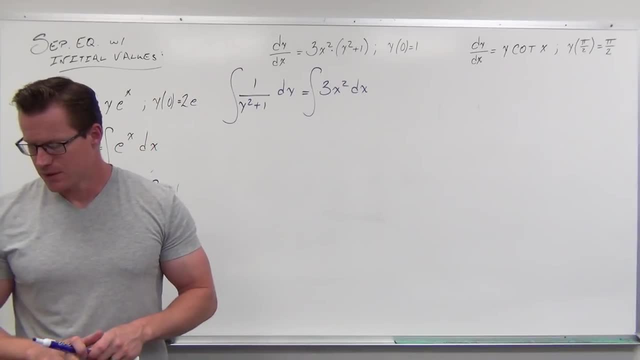 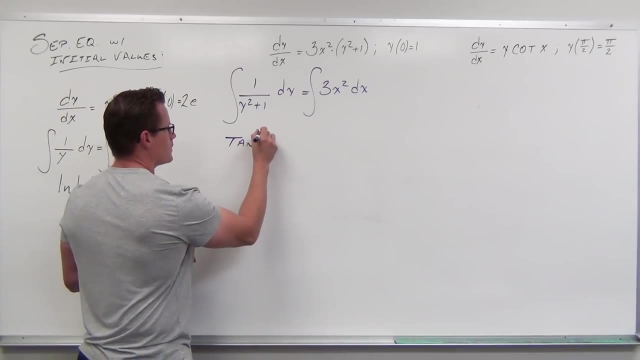 You can do a trick. so if you really want to. but if we're going to integrate quickly and effectively, oftentimes in differential equations we're using tables. So that's: tan. inverse of y equals integral of 3x squared is x cubed. 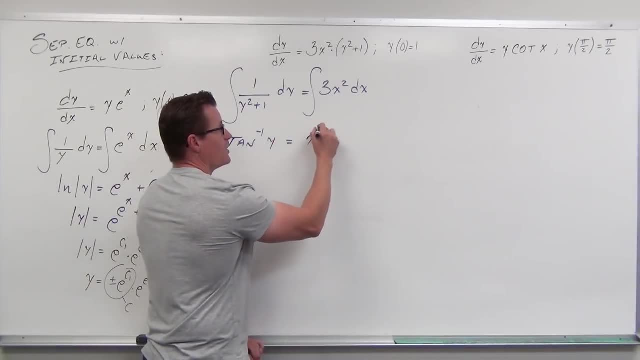 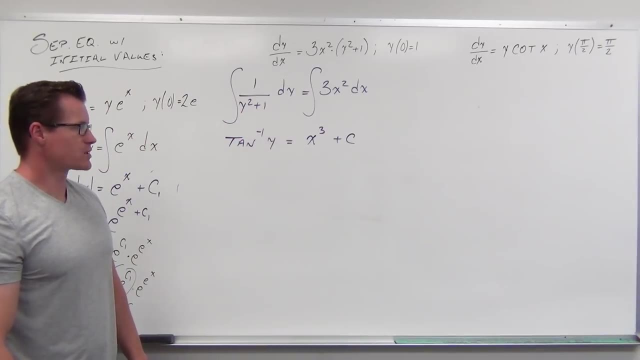 So the derivative of x cubed is 3x squared Going backwards, we get x cubed, but we'd have to tack on a constant. Now this is one of those cases where I would almost certainly plug in my initial value right here. 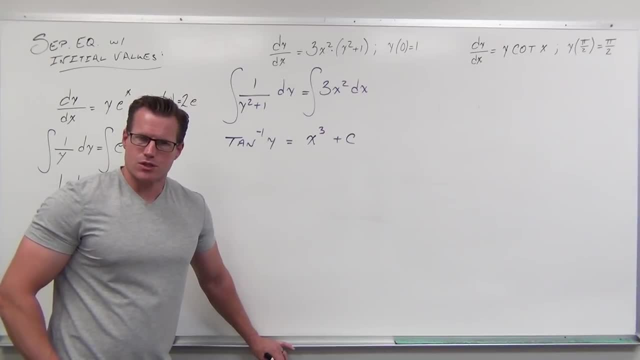 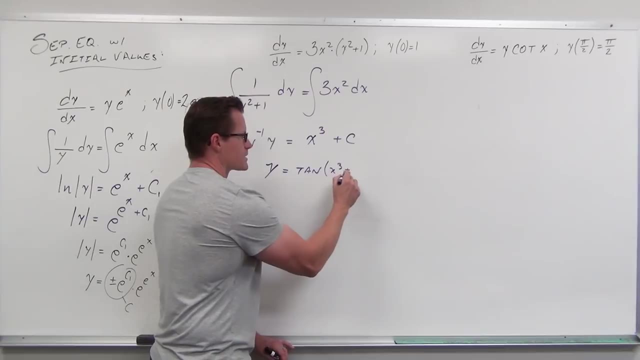 because otherwise you'd have to undo a lot of work to solve for the c. You see, if you go, y equals tangent of x cubed plus c, which we're about to do. I mean, we can solve for it If tan inverse of y equals some sort of an expression. 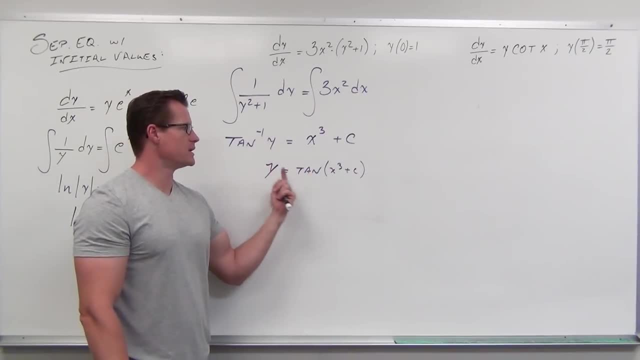 then y equals tangent of that same expression. If we start plugging in numbers here, we're going to have to do a tan inverse anyway, Do you guys get that? So if we start plugging in things now, we're going to have to go backwards from exactly where we're at here. 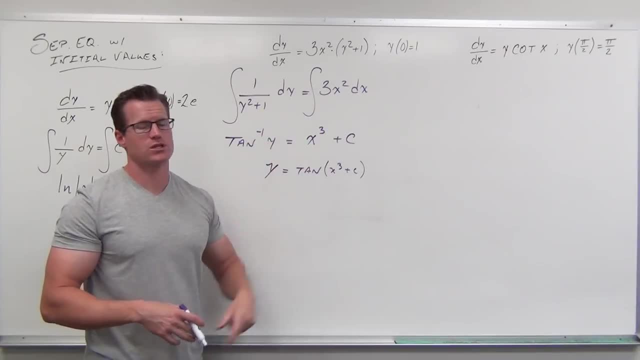 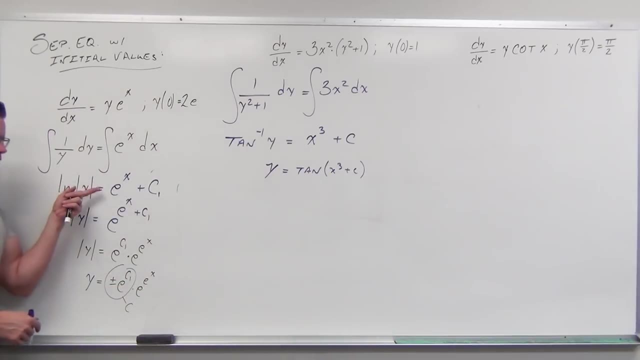 So it benefits us to plug in our initial value before we solve for y in this case. So you just have to be case-by-case specific. Is it going to benefit me to plug it in now? Well, no, Too much work, No. 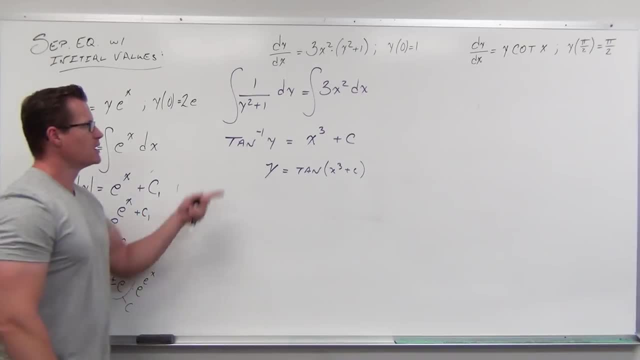 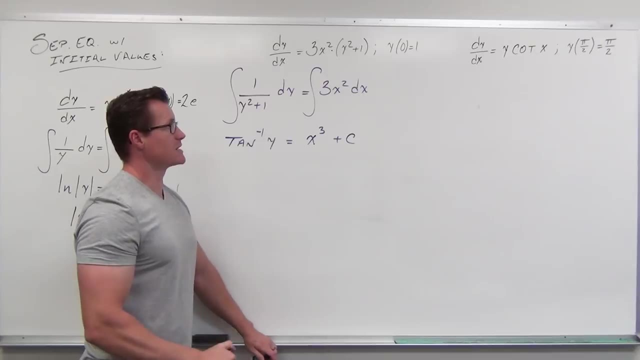 Too much work? No, Too much work. After this it looked pretty good Here. it's too much work for us to go backwards. So at this point, tan inverse of y equals x cubed plus c. Let's plug in our initial value and let's see if we can solve for c. 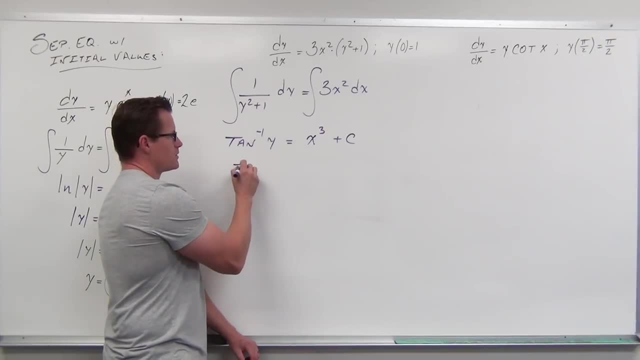 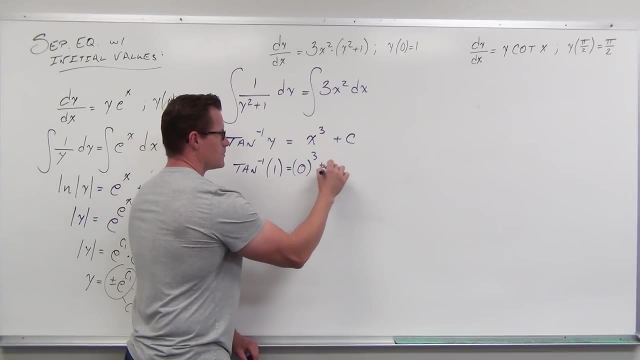 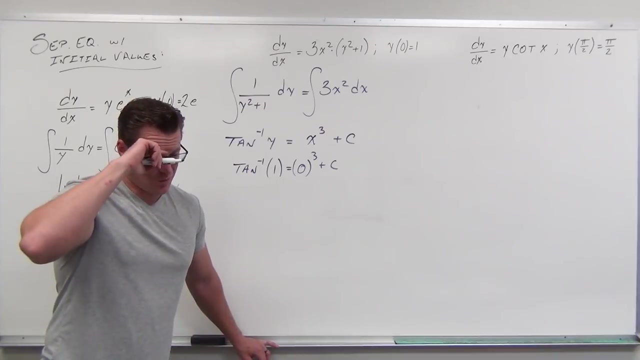 So y of 0 equals 1 says that y is 1 when x is 0. That's pretty nice, because all we have to figure out is how much tan inverse of 1 is, And that says what angle, when you take tangent of it, gives you 1?. 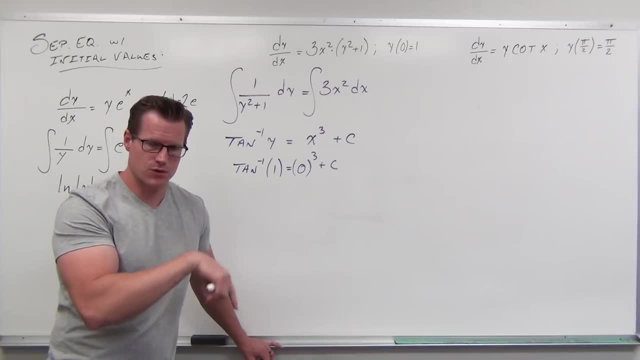 So tangent of what angle gives you 1 in the first quadrant, if you can? Well, that's going to be pi over 4.. Tangent of pi over 4 is 1, so tan inverse of 1 is pi over 4.. 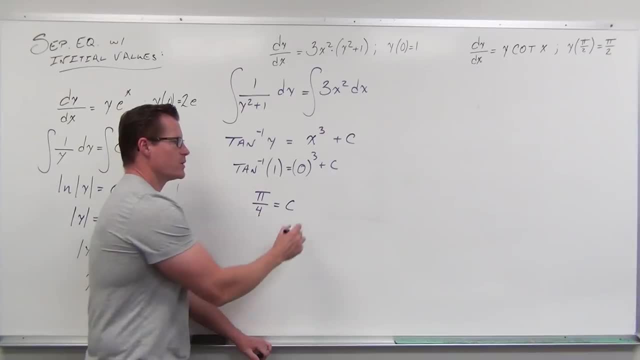 Pi over 4 equals c. And now when we plug in our initial value, we're going to have to plug in our initial value And now when we plug that back in, so we're going to get that tan inverse of y equals x cubed plus pi over 4.. 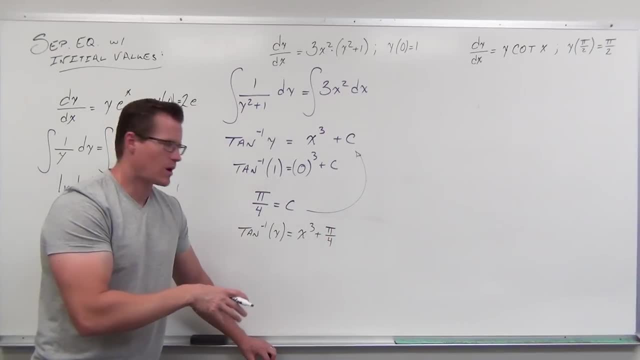 That's a little bit nicer for us to go from that point rather than get to y equals a tangent and then have to go backwards to find c anyway. So if you find yourself going backwards a lot, plug in your initial value sooner If you find yourself doing well. 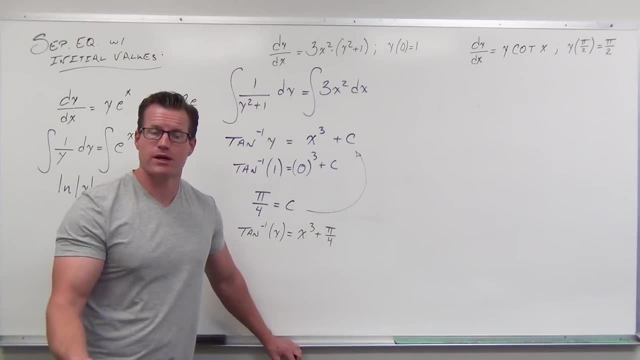 Way too much work to solve for your c. plug in your initial value later in that problem. So it really depends on what problem you're on whether you plug in your initial value early or later. A lot of times it's plugged in before you solve for y. 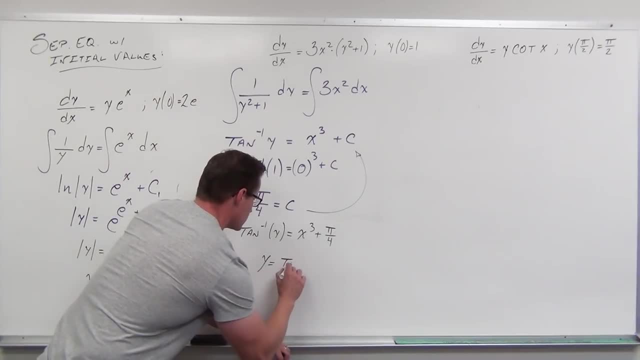 Sometimes it's not So. tan inverse of y equals some expression. That means y equals tangent of that expression: x cubed plus pi over 4.. We don't have a plus anymore. We used that, We used our point to say this narrows it down. 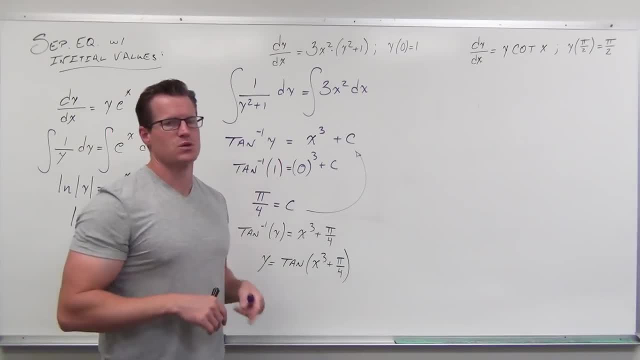 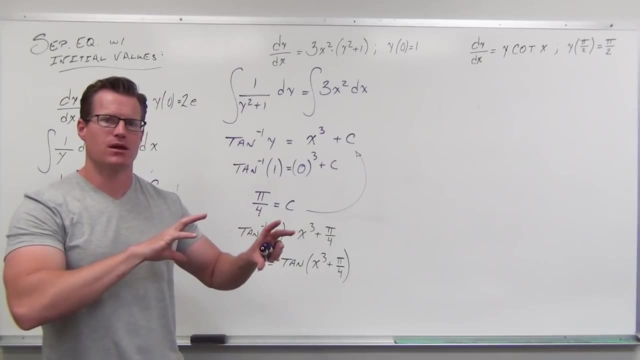 Instead of a general solution with a plus c, we have a specific solution that would go through that point and still satisfies our differential equation. I hope this is making sense to you, that you get that I'm not really teaching you anything new as far as a technique of integrating or anything like that. 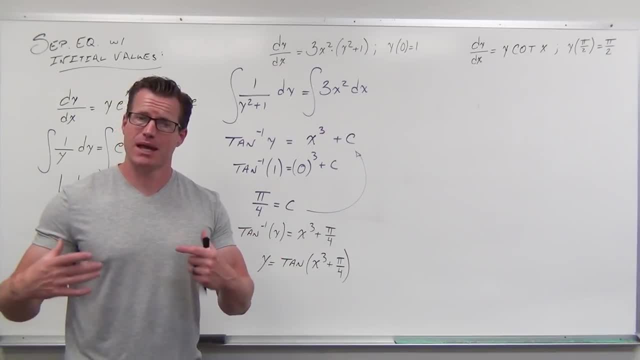 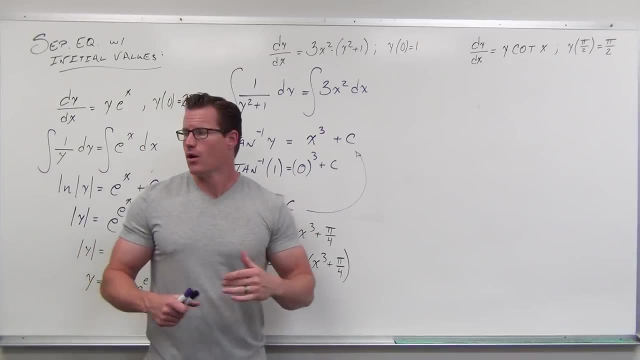 What I'm teaching you is where you should plug in your initial value And it depends on whether or not you'd have to go backwards. So if you solve all the way for y, go backwards to find your c or not. So sometimes it's easier one way or another. 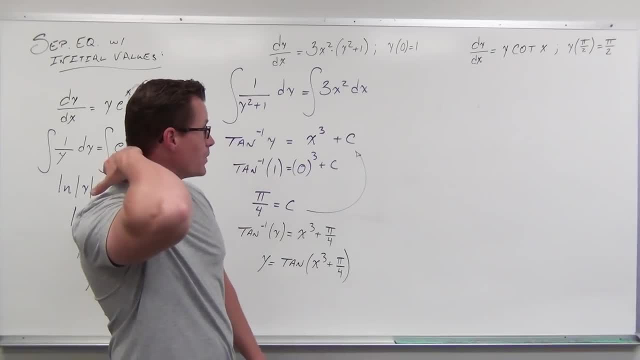 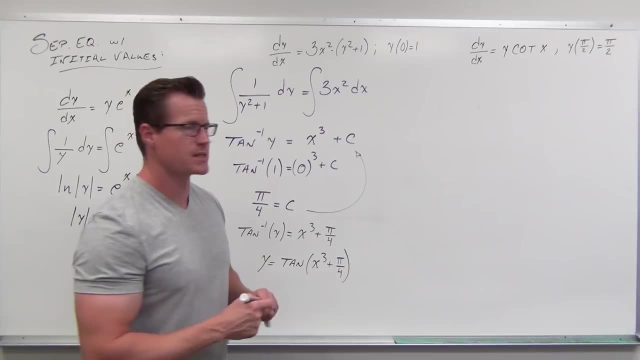 Let's do this. This last one- I'll give you three more that I would like you to pause and try on your own. So here we have a derivative of y with respect to x equals y times cotangent x. That looks pretty good because it's a product. 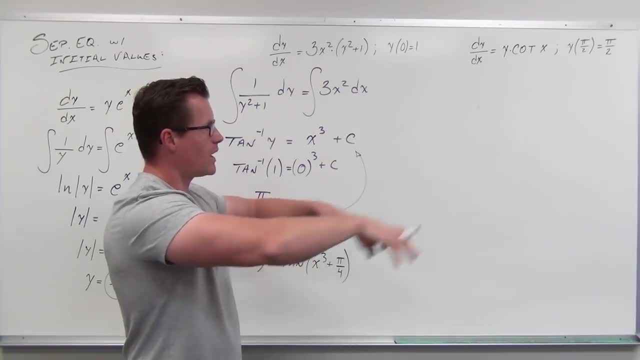 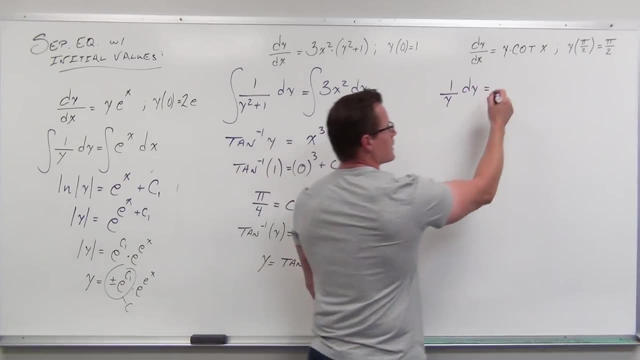 Let's group our x's dx on the right side, our y's dy on the other side. So 1 over y dy equals cotangent x- dx. We have an initial value we'll take care of in just a little bit. 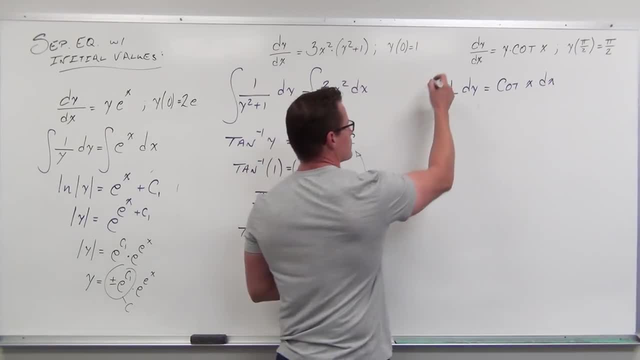 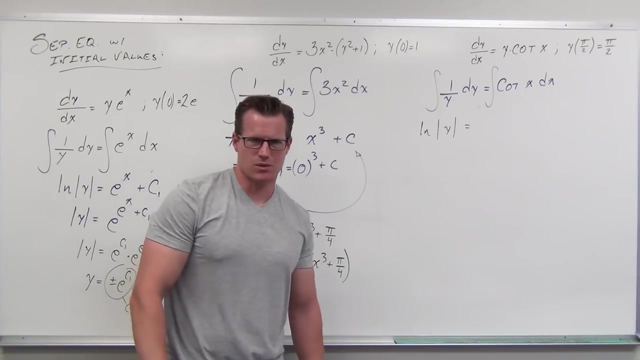 Now we're going to integrate. On the left-hand side we get natural log absolute value of y. lots of times On the right-hand side you go man cotangent x. what in the world is that? Well, let's use our integration tables. 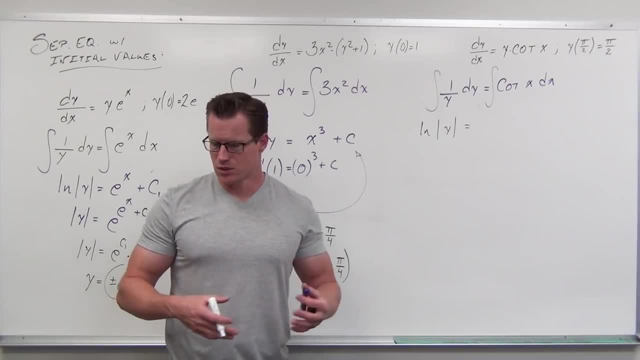 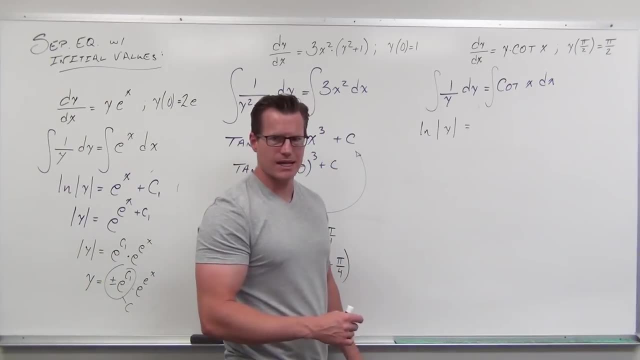 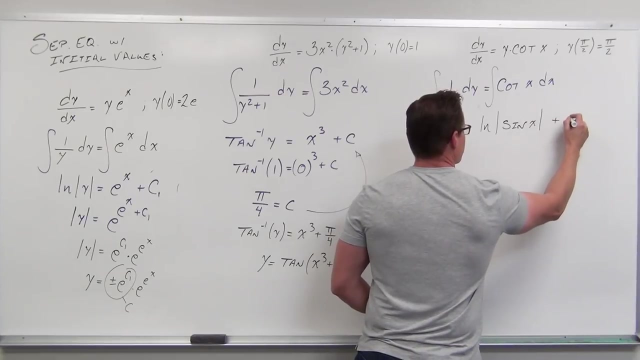 So instead of reinventing the wheel here, these are all techniques from Calc 2, but we all have them kind of down. So I'd look that up and say, okay, that's natural log, I'm going to go with sine x and we're going to get some sort of a constant out of that. 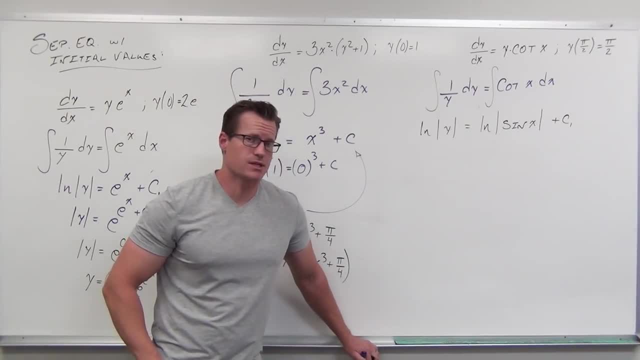 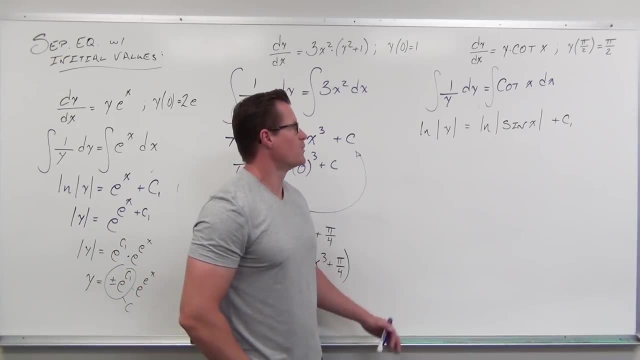 So natural log of absolute value y equals natural log of absolute value sine x plus c. Let's see what we can do with that Now, because we have a lot of- we would have potentially a lot- of work to do to solve for c right now. 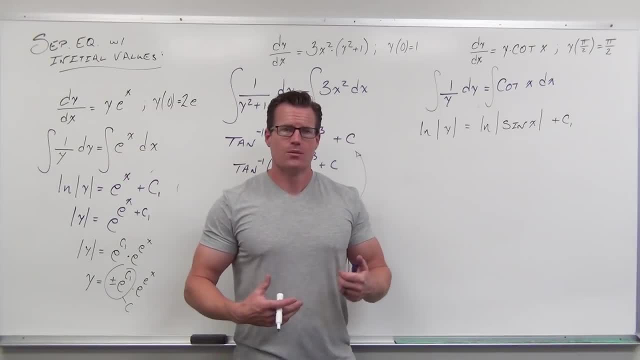 I'm going to use the same technique I had here. So you're going to find that Plugging in after you wrap up all your e to the c garbage- if you have a lot of ln's- is a technique I'm going to use a lot. 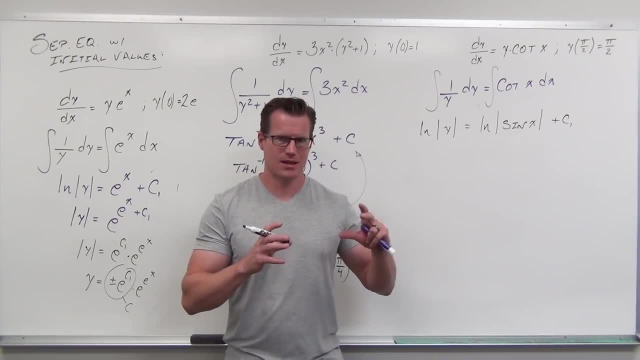 So I wait on those natural logarithms until I get that arbitrary constant of c sub 1 into being like a bigger expression, where I wrap it up into a bigger c and then I'll plug in my initial value. That works for me very well. 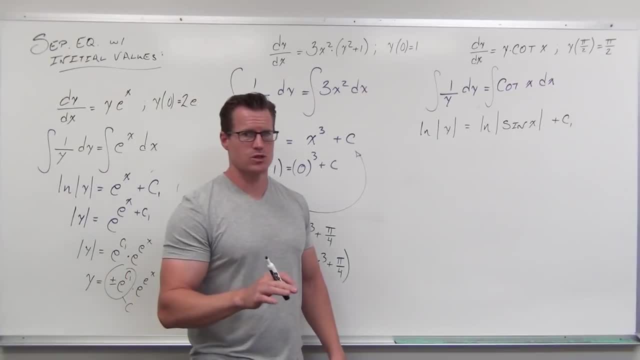 If I don't have that most of the time, I'll plug it in as soon as possible. So now we're kind of narrowing down. Now, when do I plug in that initial value? Well, if we have a lot of exponentials going on. 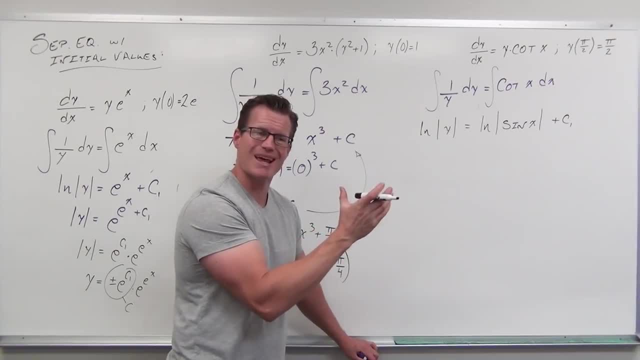 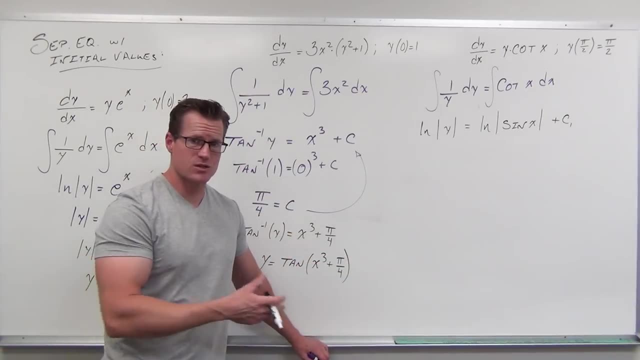 where I can start wrapping up a- c in a bigger expression. that saves me some work, saves me going through that expression again. If I don't have that well, I can solve for plus c as soon as possible and then solve for y with an actual number instead of a c. 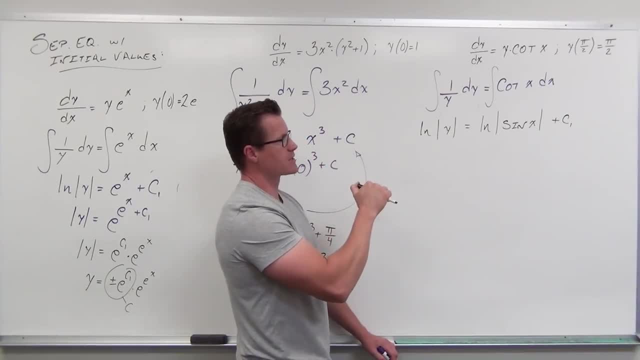 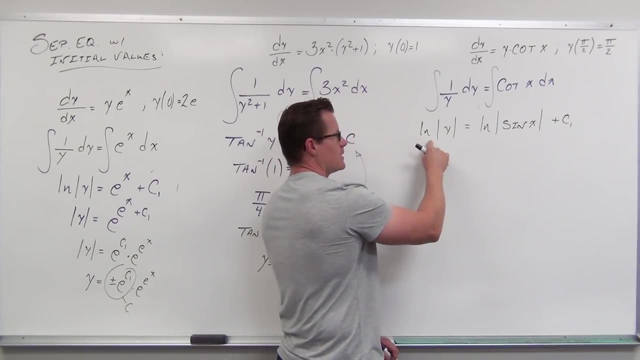 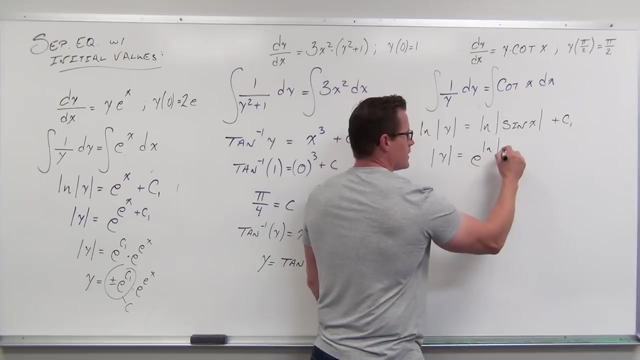 Let's see what I mean here. So ln absolute value y equals ln absolute value sine x plus c1.. Well, we know that we're going to have e raised on both sides. So Exponential to exponent equals argument. So e to the ln absolute value sine x plus c1.. 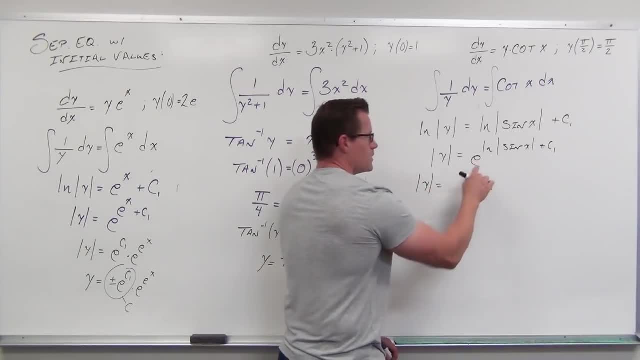 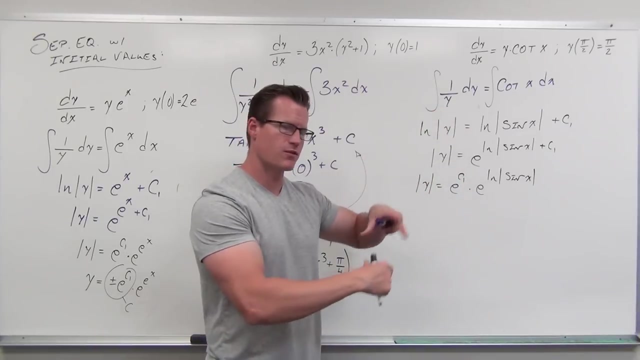 We've done this many times now, So I'm going to separate this into a product of common bases. And we know that when you compose two functions that are in a particular order, versus, they eliminate each other, they undo each other. So I'm going to do two things now. 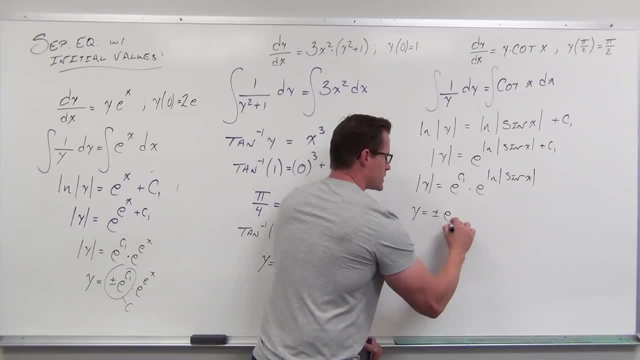 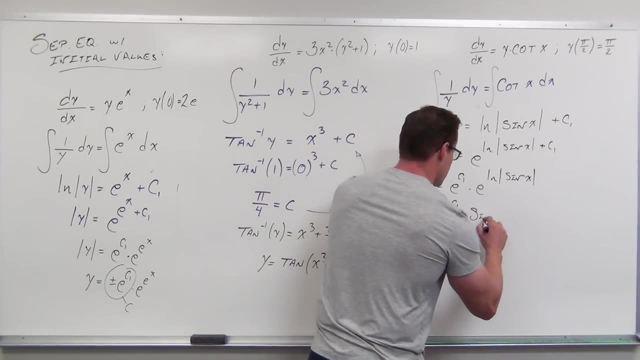 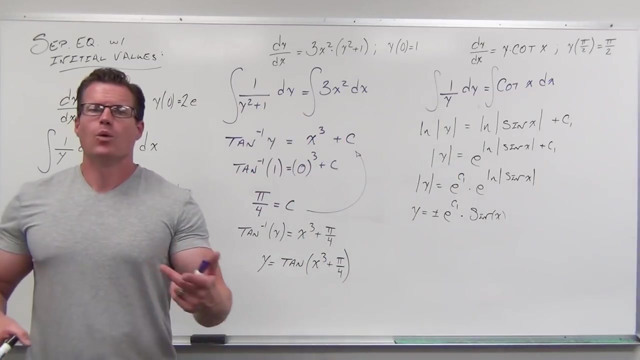 Absolute value of y. I can write this as: y equals plus or minus e to the c sub 1.. I can also eliminate my e and ln and just get sine x Next up. what would you do here? So if we had? if we had this, like on a test or something, 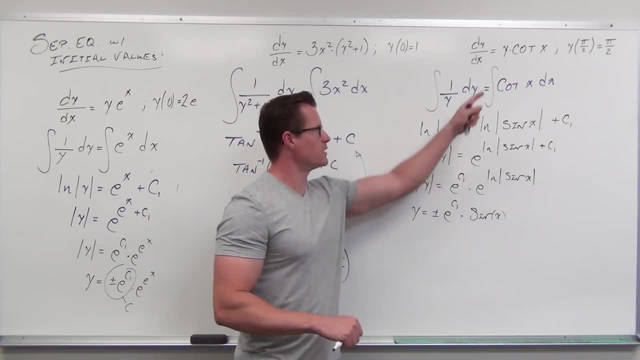 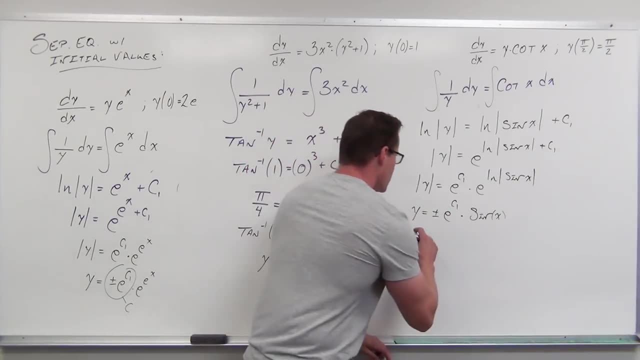 would you wrap this up Or would you plug in your initial value? If you plug in your initial value, now notice all the work you have to do to get to that. c. That's, that's not very fun If I wait just a moment and say I'm going to call all this stuff c. 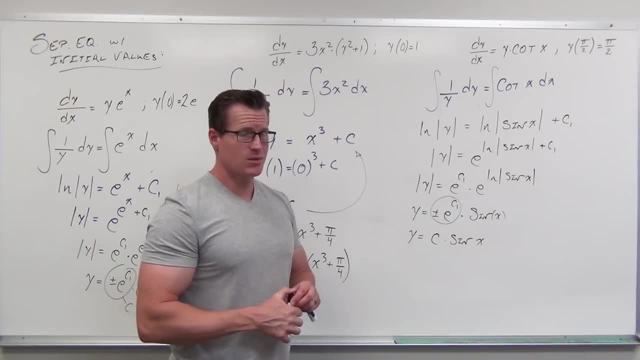 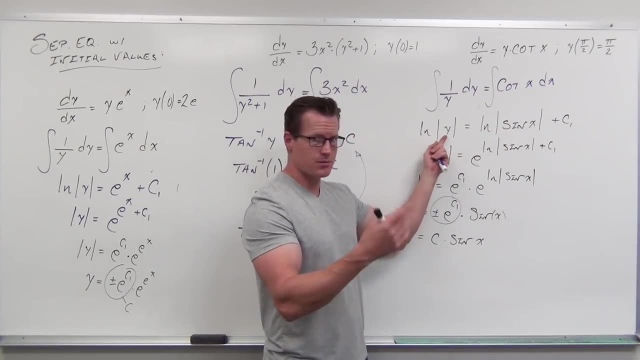 Yeah, we'll have to go backwards a little bit, but it's a lot easier to see what that c is, because even here we have a lot of ln's going on to unpack all that garbage. We have to have ln of some expression. however, two 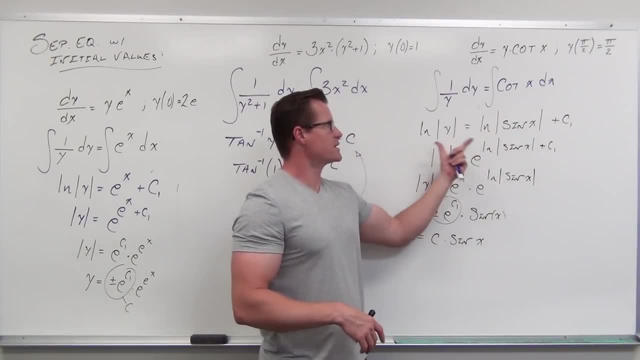 So sine of pi over 2, ln of that Now, is that a big deal in this case? No, they're both pi over 2's. You subtract them and you get what you want out of that. But here it would be a little bit nicer. 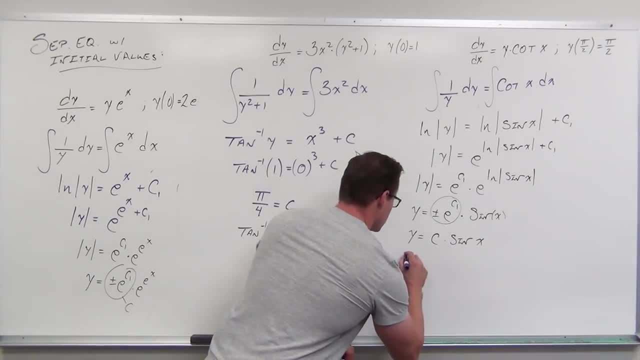 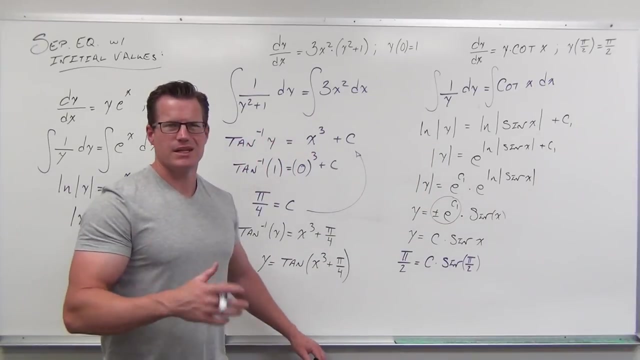 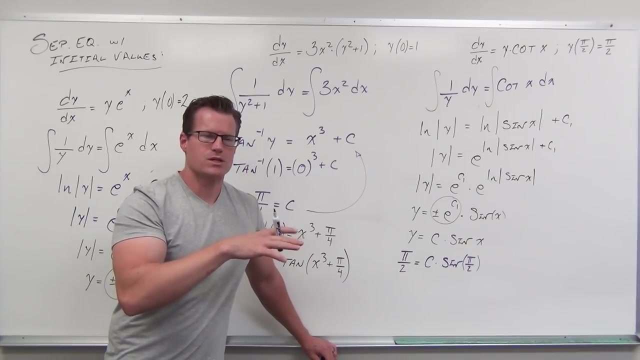 So this says that y is pi over 2 equals c times sine of pi over 2.. You need to know what sine of pi over 2 is. So sine of cosine and sine, sorry, sine and cosine of our normal, well typical angles are. 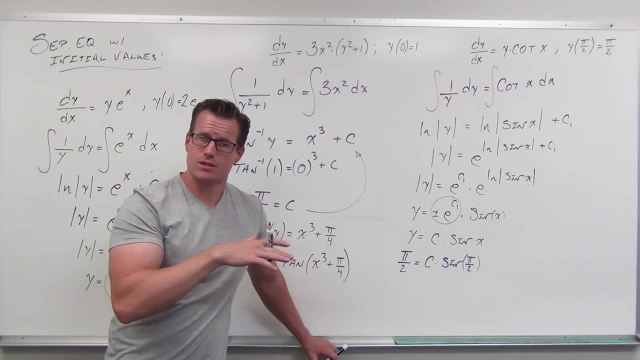 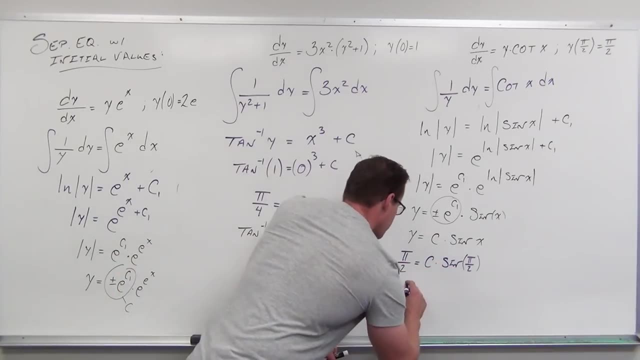 really important to have memorized. So sine of 0 is 0, cosine of 0 is 1, sine of pi over 2 is 1, cosine of pi over 2 is 0. So I know that that's 1, which means that pi over 2. 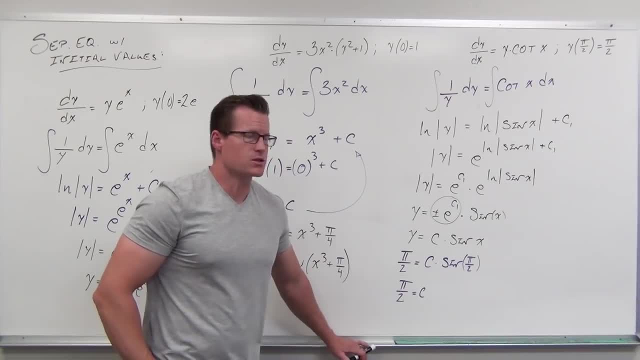 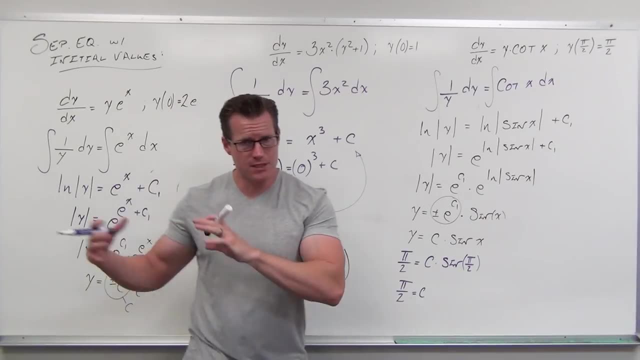 is equal to c. That would have been. that's a lot easier than plugging in first. If we plugged in here we'd spend a lot of time solving for c. But with exponentials oftentimes it's easiest to wrap up that e to the c sub 1 plus or. 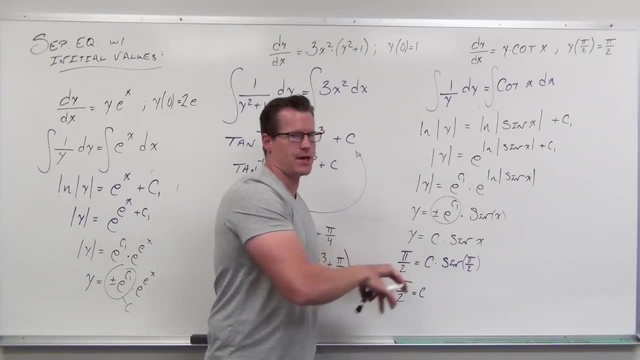 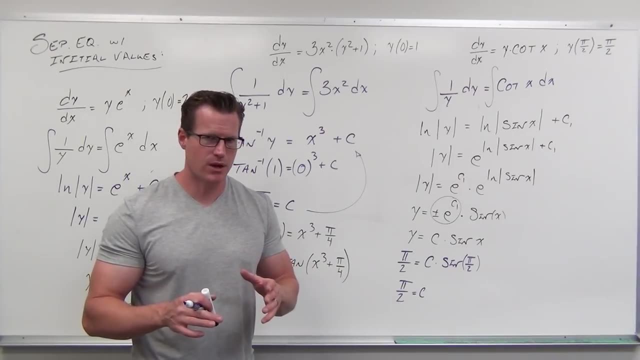 minus as an arbitrary constant and then, right after that, plug in your initial value. That'll save you some headache. So I know that it's. hopefully it's not ambiguous as to when you plug it in right now With exponentials, if you can. 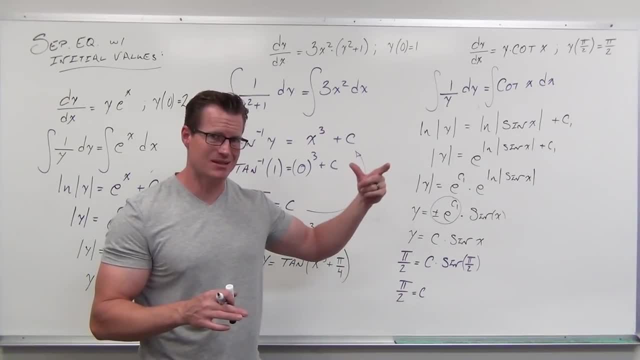 wrap up the plus c. if you know you're gonna be able to wrap up the plus c in something like a, c, e to the c sub 1 exponential, or a plus and minus that, or changing your sine to get rid of. 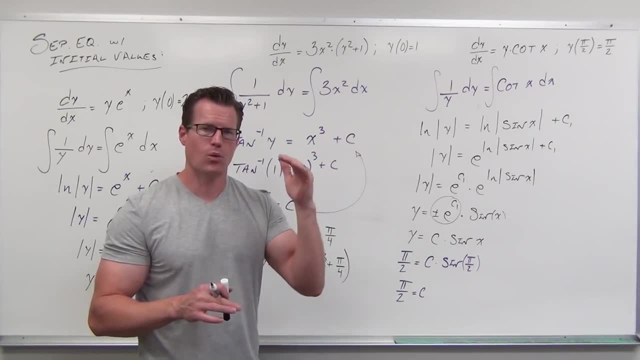 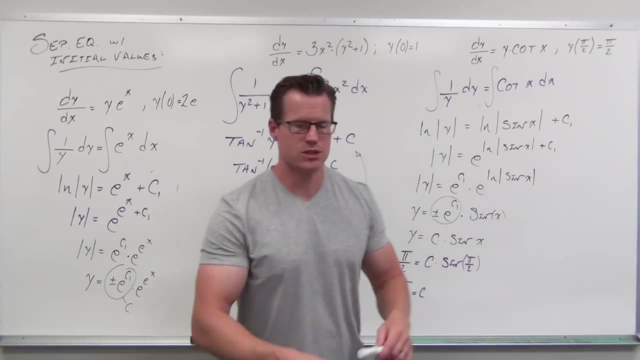 constants by wrapping it up into a bigger arbitrary constant. wait to plug in your initial value. If you know you're not gonna be able to do that, plug it in as soon as possible. So that's how I approach these problems. So here we're. 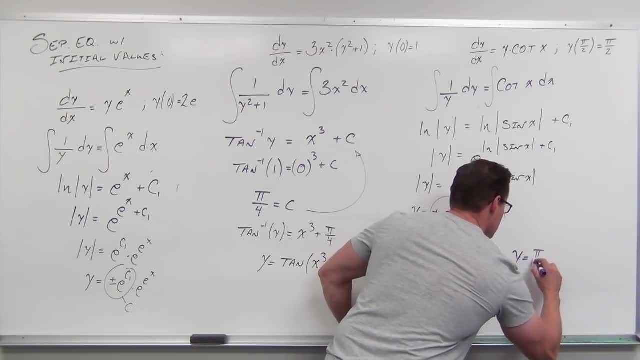 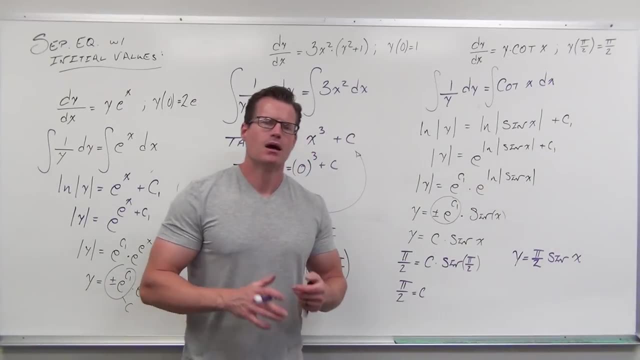 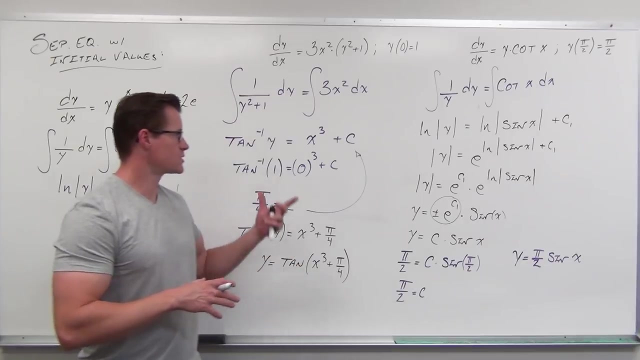 almost done. All we need to do is write this as: y equals pi over 2 sine x. done, That's it. Are you getting it? Are you understanding why I'm plugging in my initial value, sometimes soon and sometimes not soon? 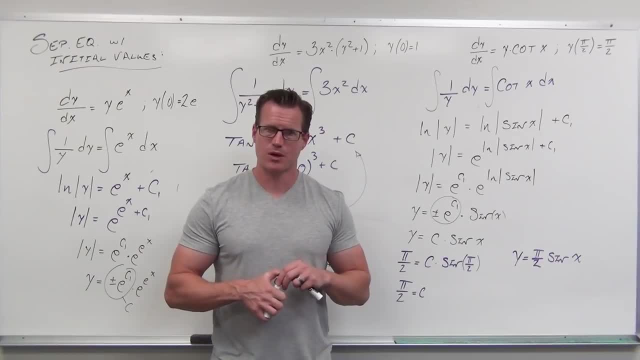 It'll also do with the form of our problem. If we're able to wrap up our constant into something larger like that, this becomes a bigger c. if you will, It's best to wait. If you're not able to do that, it's best to do your initial value. 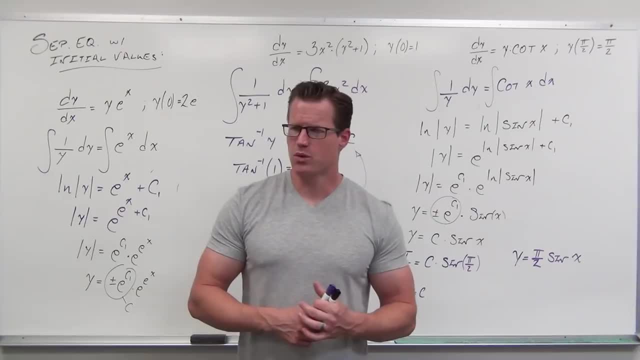 sooner. We have three more. I'm gonna go through pretty quickly, but when I write them on the board, I'd like you to pause the video and try them on your own, See if you can work your way through. Think about what you're going to do next, If you're. 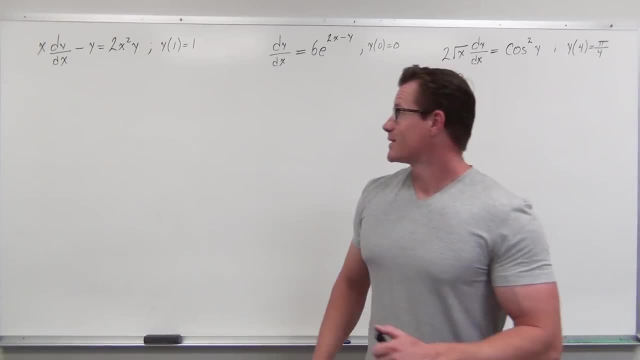 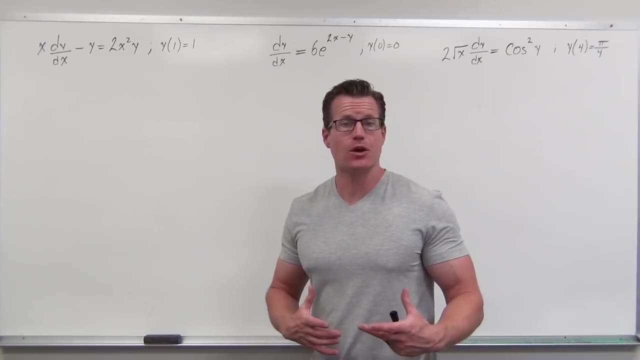 able to do that. think about when you would plug in that initial value. Okay. so if you want a challenge, I would say, try these three. There's some weird stuff going on, which is why we're doing them, and I'll show you exactly how to go. 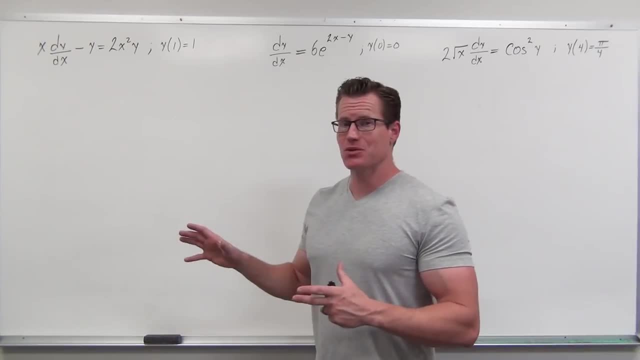 through and how to approach this sort of a problem. But if you'd like to, here's the hints. I'm gonna give you the hints and then I'll go through them pretty quickly, but I'll be explaining everything for you. So first one that can: 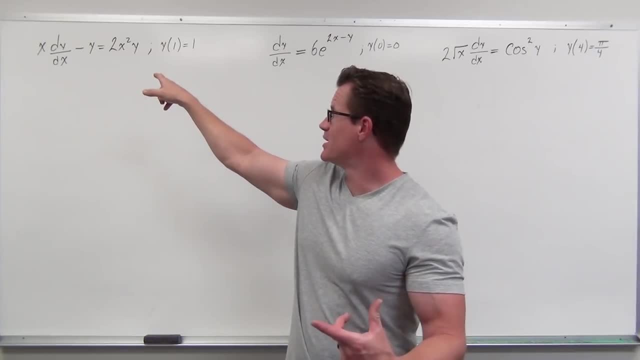 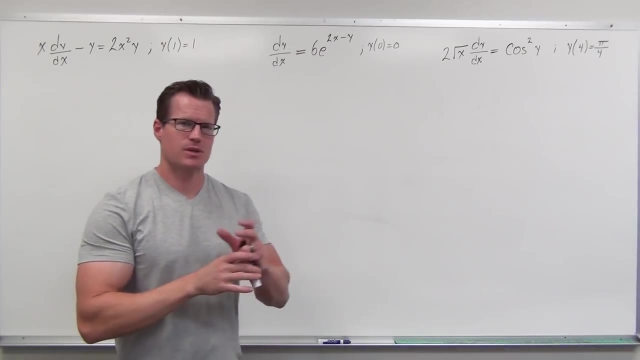 be written as a separable equation, but you've got to add the x and factor. So see if you can factor that this one. Well, that's an exponential with exponents that are subtracted. See if you can separate the exponent. Last one, actually. 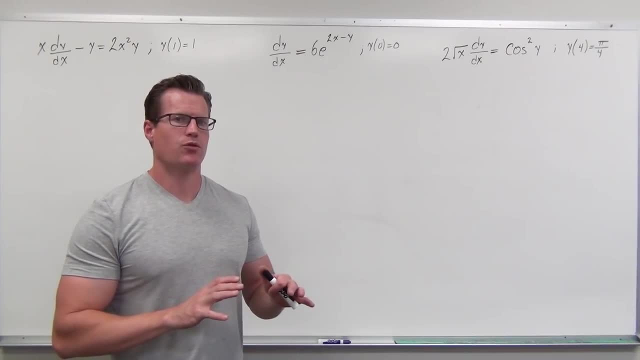 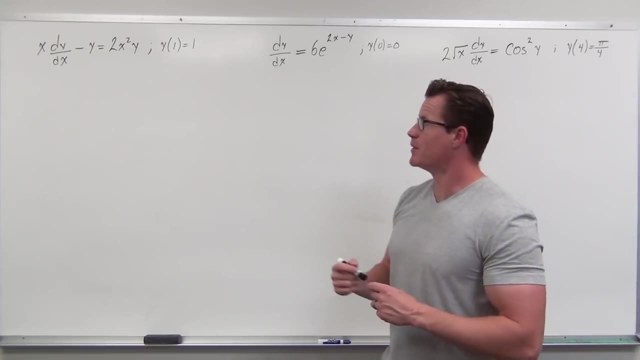 last one's pretty good, so last one's not not too bad. It's already set up pretty well for you. So if you want to challenge, see if you can do these ones, I'm gonna get started right about now. So first example: Can we write it a separable equation? That's our primary. 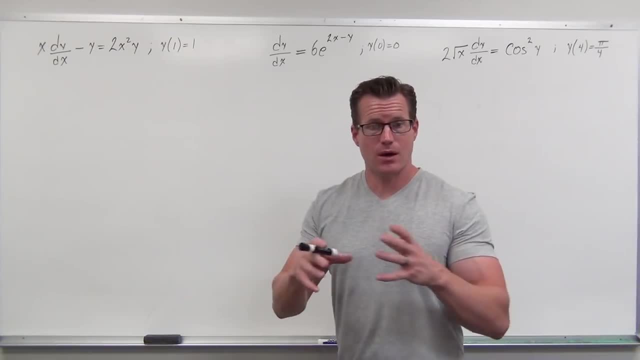 goal right now because, well, honestly, it's the only technique you know. But other than that, that's okay, Since it doesn't really add any time. Other than that, it's the easiest technique that we have. It doesn't involve a lot of setup, which some of 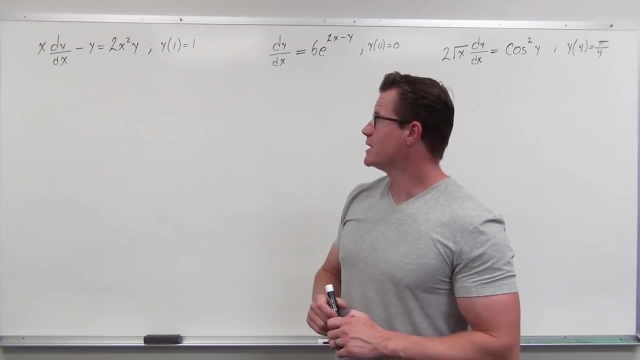 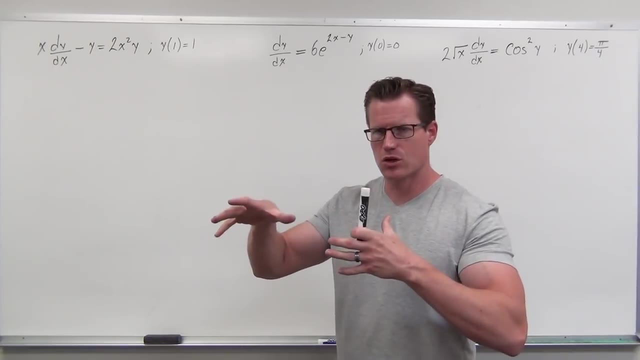 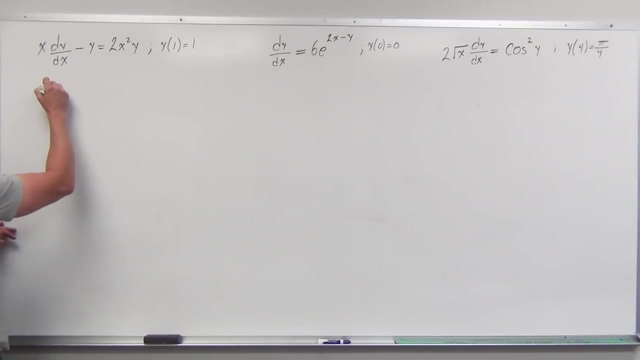 the other techniques do involve. So here let's see if we can. well, if we have more than just two big terms, one on each side, we're going to need to group our terms and see if we can factor. So in this case that involves adding y and seeing if we can factor out, and of course we can, We can. 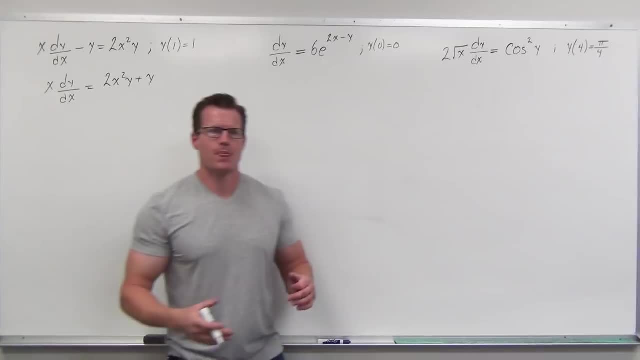 factor GCF of y, What that's doing. what the idea is is: you need products, right, So you need just factors that are multiplied together. If you have more than that, if you have stuff that's being added and subtracted, you need to be able to factor in order for this technique to work. 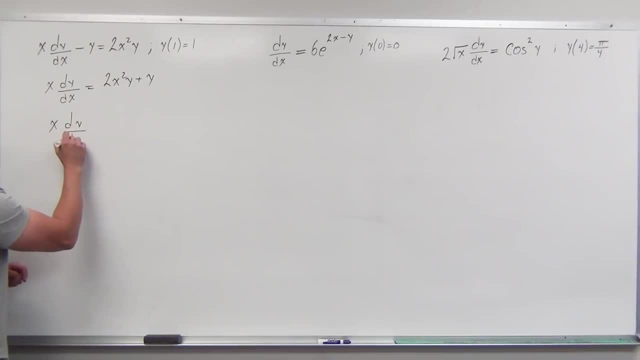 That's looking pretty good. We factor out our y, we get 2x squared plus 1.. Now we can leave this divide by x, divide by y and move our dx. So we can write this as our variables grouped together. 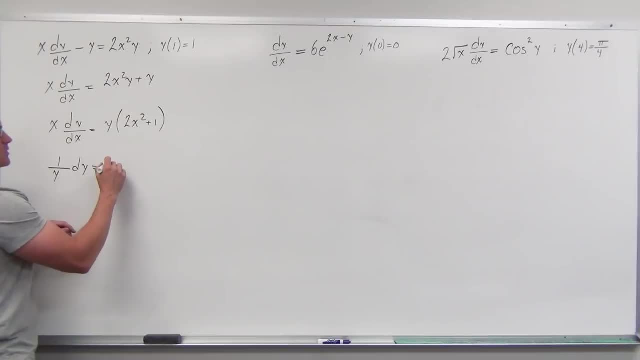 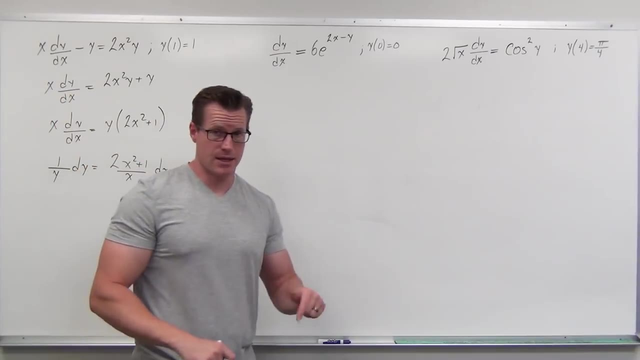 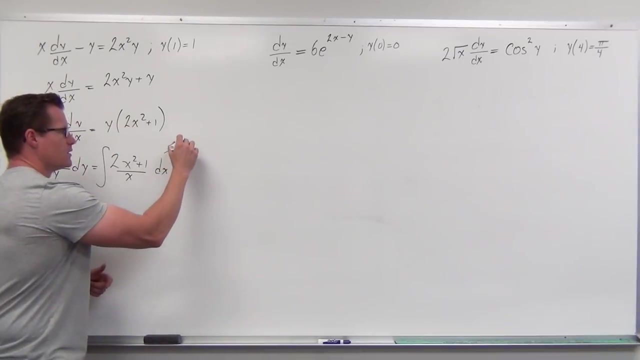 1 over y dy equals 2x squared plus 1 over x dx. Now we're ready to take that integral On the left-hand side. pretty straightforward On the right-hand side, notice that we can separate this. If we separate these fractions, we get: 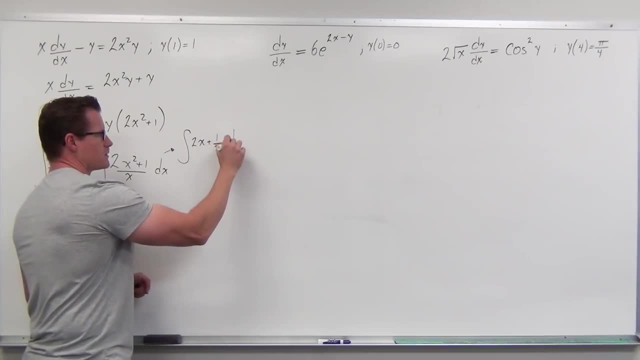 2x plus 1 over x dx. We separate this, we get 2x squared over x. that's 2x. 1 over x is of course 1 over x. So when we do our integrals, ln absolute value of y is pretty good. This is just x squared. 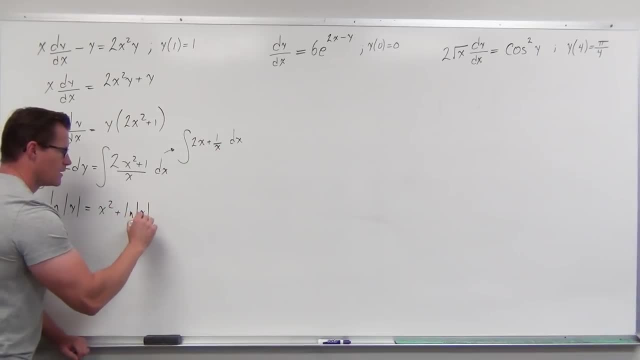 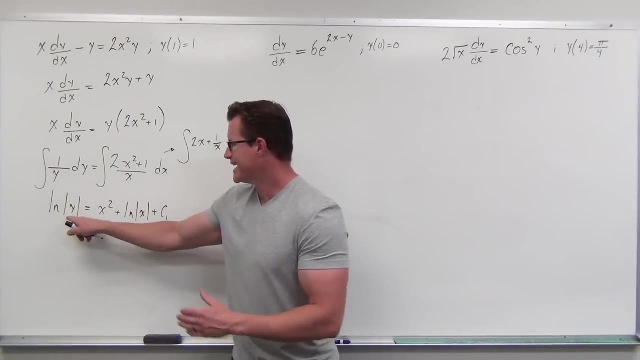 this is ln absolute value of x, and then we get this plus c1.. Notice what's happening. What's happening is: I am going to have e to all this side. I'm going to have an e- c1.. I'm going to. 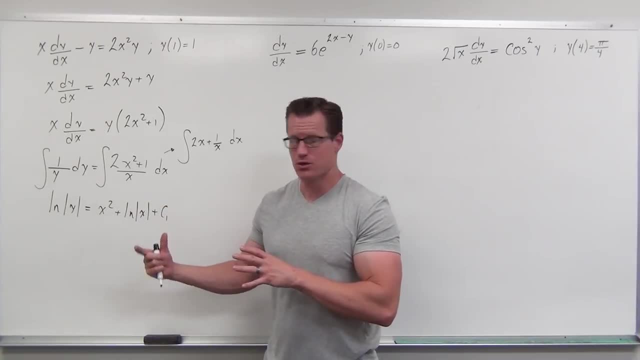 have a plus and minus. I'm going to wait to plug in my initial value Now. could you do it now? Absolutely, But it gets a little tricky- what you leave in terms of e and what you don't. So right now I'm going to and either way you want to go, you'll be fine. 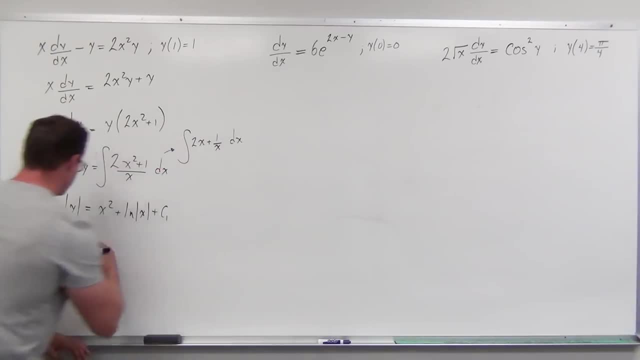 But I'm going to wait just a little bit. What I'm going to do is understand that an exponential undoes logarithms. I'm going to have e to the x squared plus ln, absolute value of x plus c1.. I'm also going to split this up. I know that. 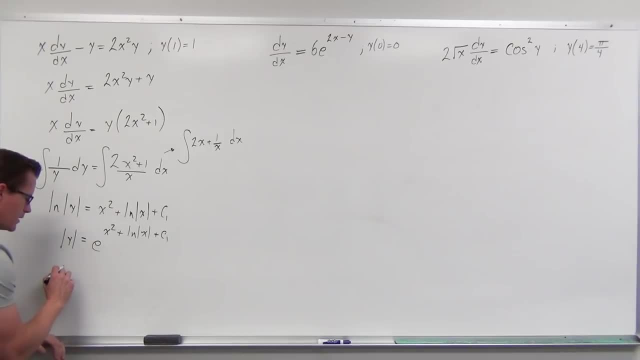 exponents being added came from common bases being multiplied. So I'm going to put my e to the c1 first. I'm going to have c1 plus ln absolute value of x plus c1.. I'm going to multiply. excuse me, multiplied e to the x squared and e to the ln absolute value of x. 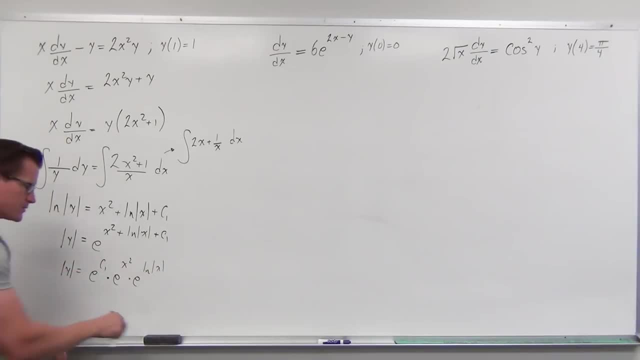 Well, that's great because we can take this absolute value of x, which is going to have a plus and minus in it, and a plus and minus right here, and say let's just wrap all of that up with a plus and minus e to the c1.. 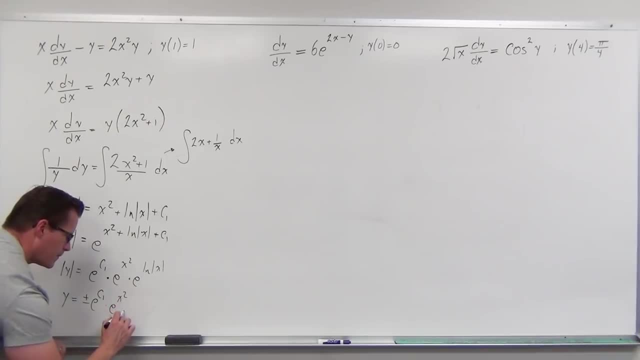 We'll have an e to the c1.. We'll have an e to the x, squared, But e to the ln. x gives us just x. That's great, Actually almost done. So if we rewrite this, what we're going to do is we're going to group. 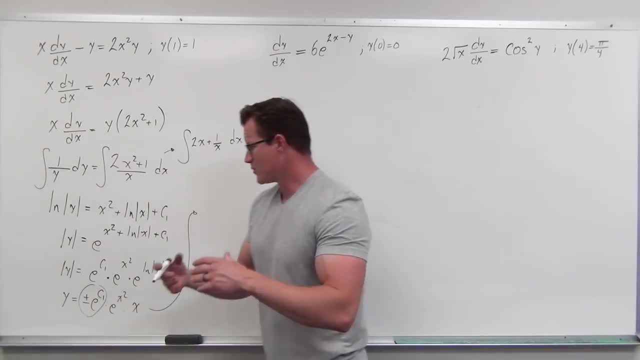 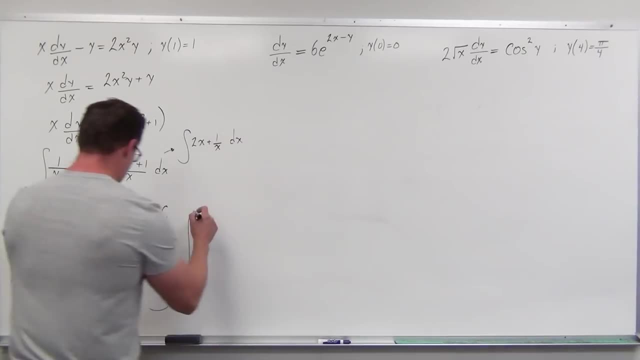 all of this and say: hey, you know what? That's still a constant. c sub 1 is a constant. e to the: c sub 1 is a constant. Whether you have positive or negative, you're still going to have a constant. Let's call that big C. So y equals c. 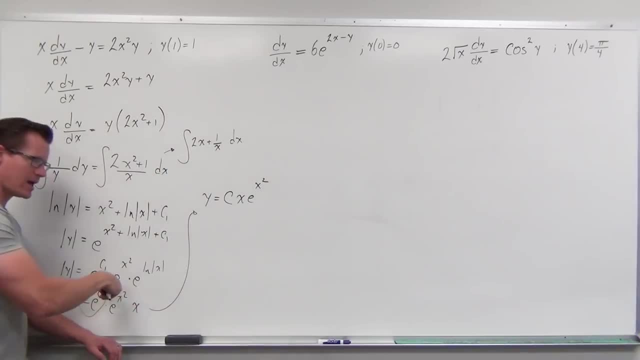 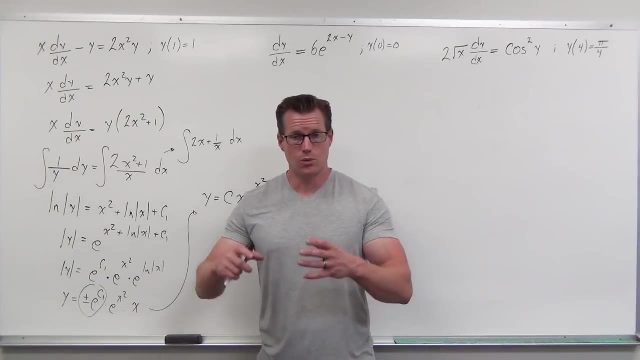 times c, c times x, e to the x squared. I'm just moving my x into the front If you're wondering. well, what about the absolute value? It's wrapped up in that positive negative, So we can wrap both sides. Absolute value would just give us a positive or negative, whatever. 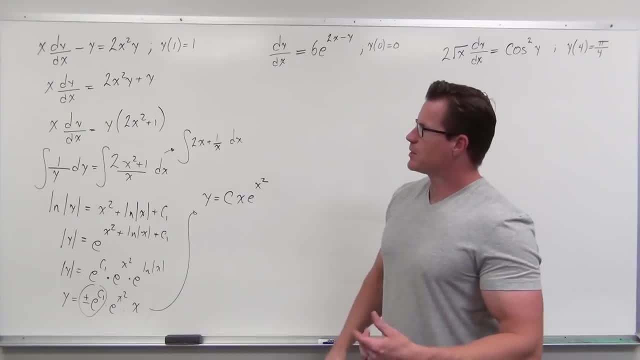 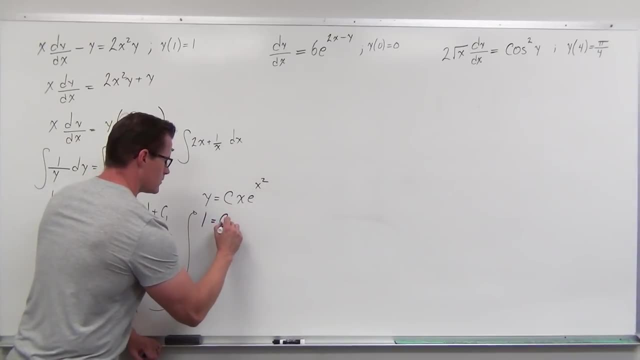 we have there. So we wrap that up and now we can plug in our initial value. So y is 1 when x is 1.. Well, what that means: c times 1 times e to the x squared that's going to. 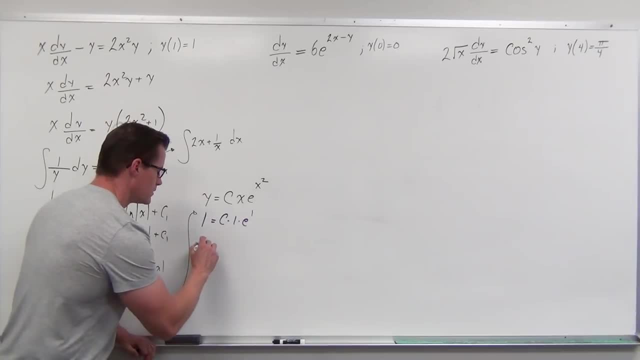 be 1 over e. So the first is just c times e. If we solve for c, we get 1 over e, which changes our solution here to 1 over e, x to the x times e to the x squared. That's not. 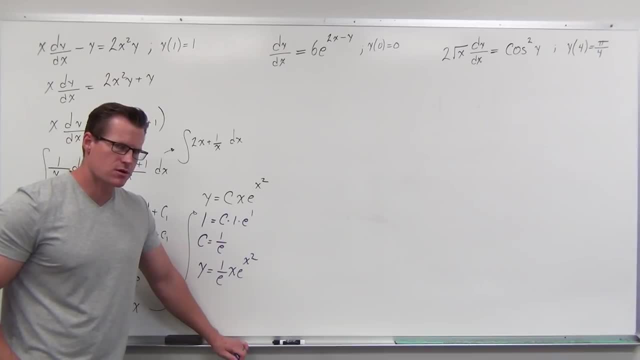 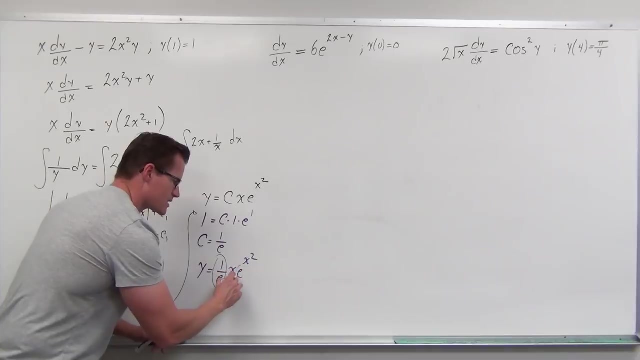 what my answer looks like in the back of the book, or if this came out of a book, or if you're doing it on a test, or whatever you're doing. That's not what it looks like. That's because of this. Many times, if you have a constant with a base, that's the same as some other. 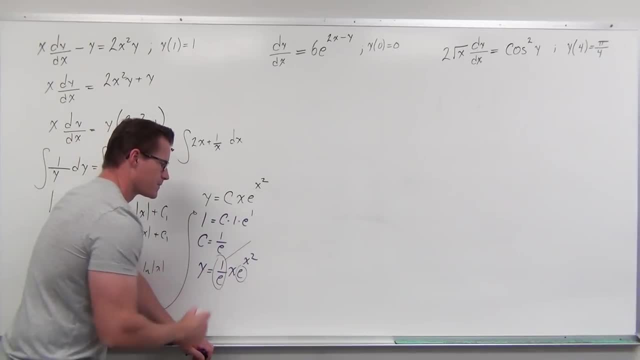 exponential that you have. we can rewrite this: 1 over e is the same as e to the negative 1.. We can do that. If we put it in the back, it's pretty easy to see that we now have a common value. 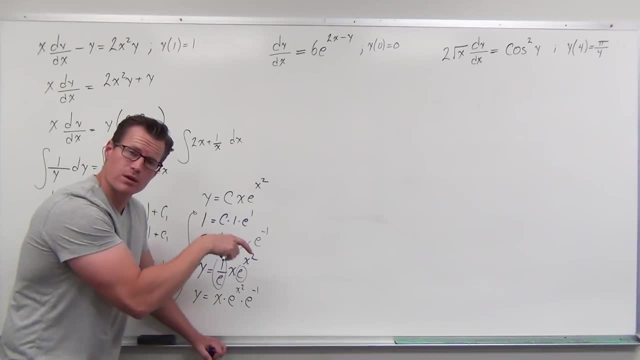 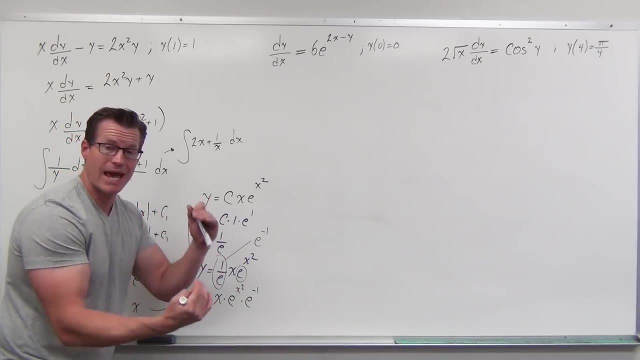 If we have common bases, which is why we wrote it as e to the negative 1, to show that we have common bases. If we have common bases, what do we do with our exponents? Let's see Multiplication of common bases. we would add our exponents, So y equals x, e to the x squared. 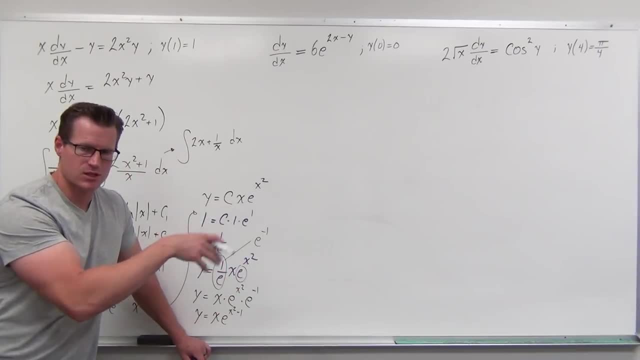 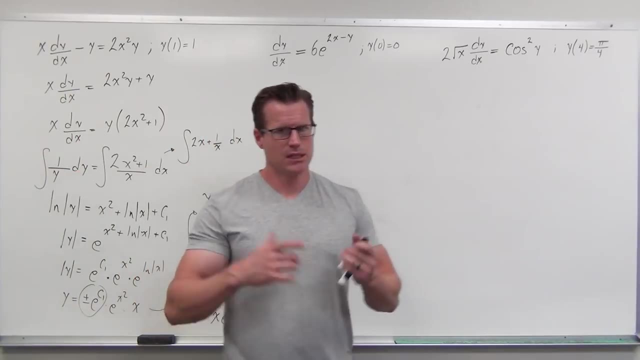 minus 1.. x squared plus negative 1 is x squared minus 1.. That's the way to approach that problem. So, same ideas, Maybe factor. If you have more than just stuff being multiplied, you're going to have to factor to create those products. 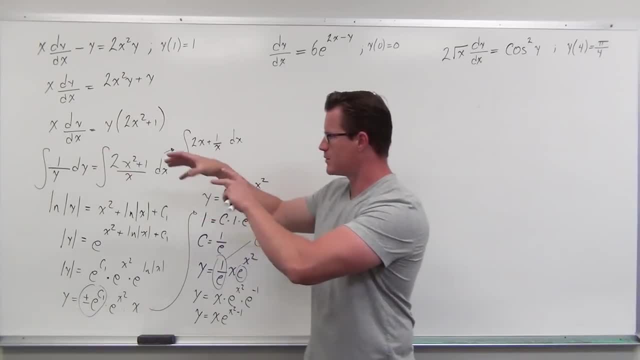 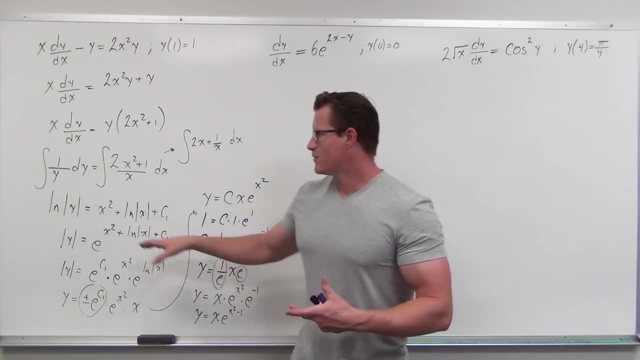 So we factored, We moved our x's and y's on the appropriate side with dy, dx. The integral is pretty easy here. And then I'm always going to follow this pattern of: if I have an ln, if I know I'm going to have an exponential over here, and it's all raised to an exponential. 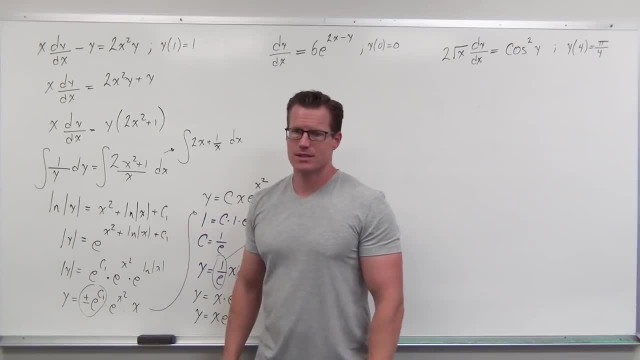 not just little pieces but all of it. and I know I'm going to get an e to the c sub 1, and I know I'm going to get a plus and minus. I'm going to wait to plug in that initial value. If not, I'm going to plug it in early. 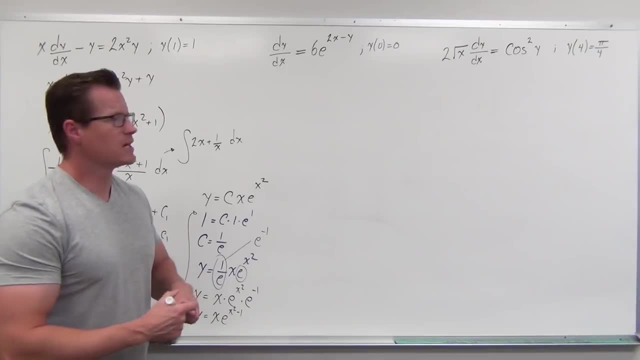 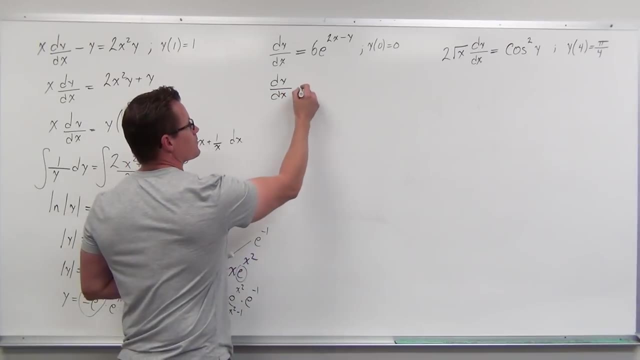 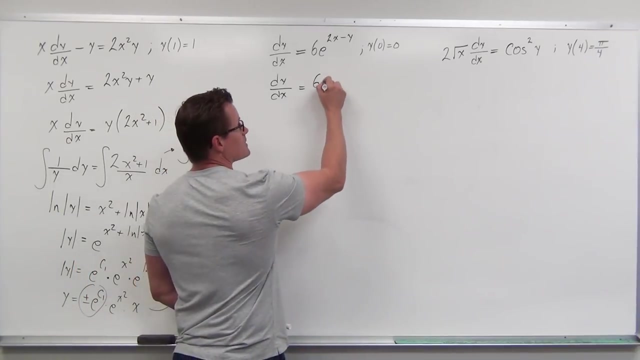 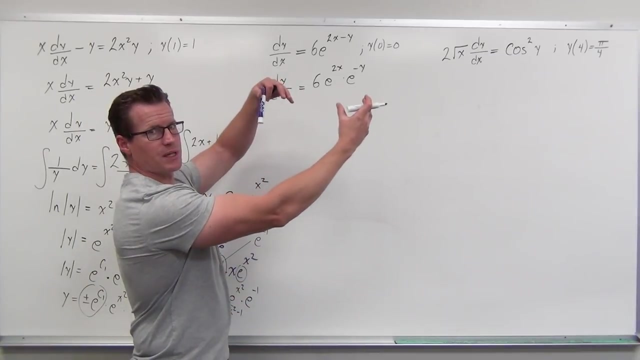 Let's check out the last two. So this next one looks really tricky. One idea here is that if you have to separate your variables, then you have to separate any exponentials that contain both your variables. which means we have 6 e to the 2x times e to the negative y If exponents are being 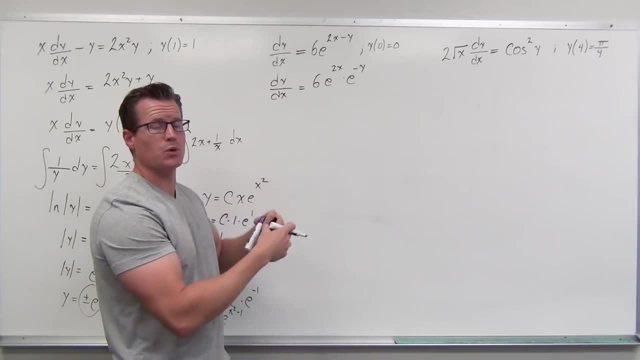 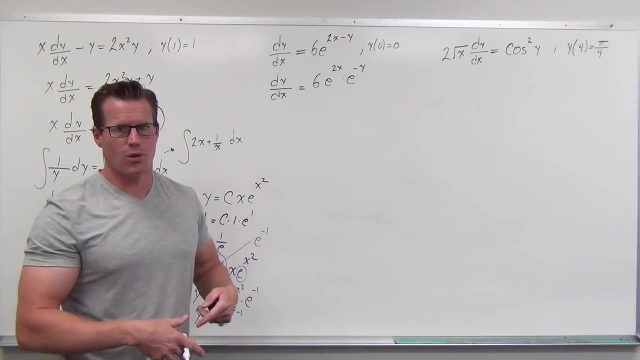 added or subtracted. we can split them up by positive or negative multiplication of those common bases to those exponents. Could you have also put e to the 2x over e to the y? Absolutely, That's fine. In fact, that might be a little bit easier for you to see. 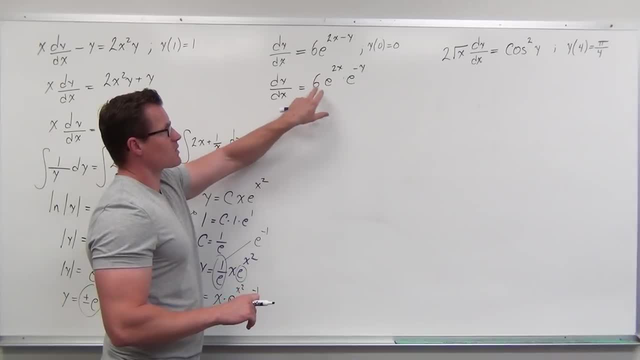 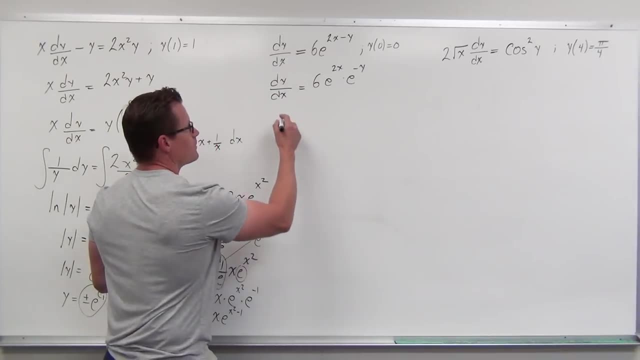 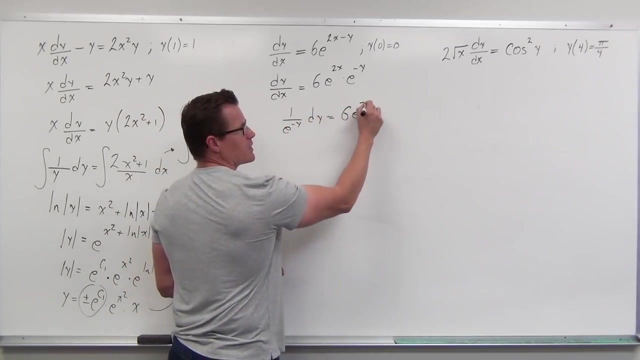 the next step. So if I've got my x's here and I leave my constants, remember that We leave our constants on the x side. I'm going to move this over here. So we would have either 1 over e to the negative y dy equals 6 e to the 2x dx Or, if you really think about it, you could. 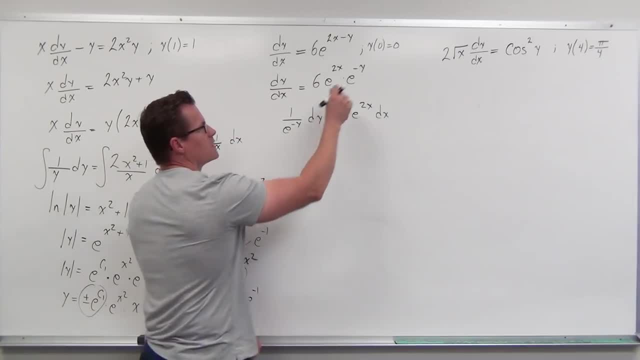 think about it. That's just e to the y, which would be what you'd get if you divided by e to the y. here You'd go: yeah, I'm going to multiply, I'm going to get e to the y. 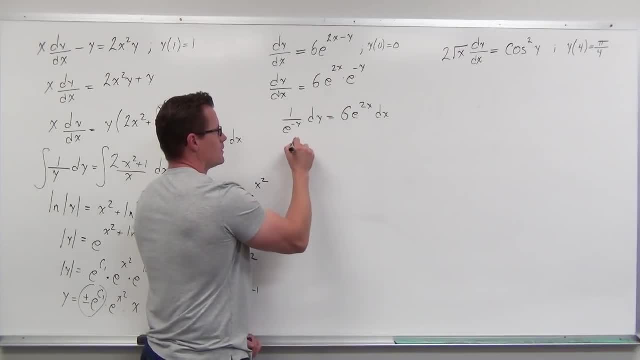 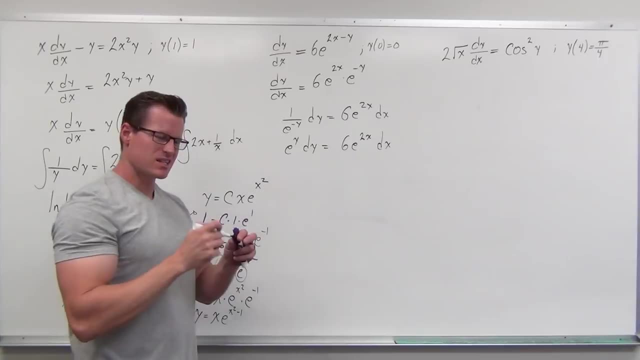 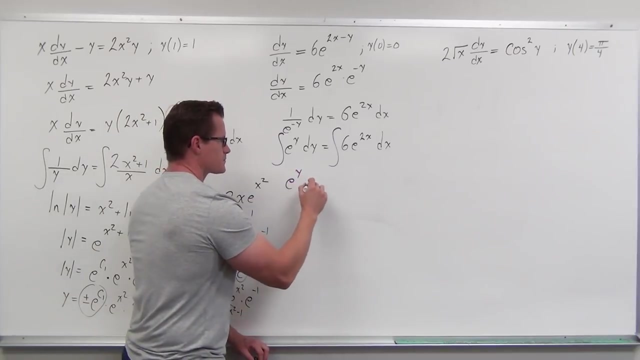 That would probably be an easier way to do it. I group my y's in dy. I group my x dx. We're ready to integrate. It's looking really solid. I love e to the y. It's just going to give me e to the y On the right-hand side, 6 e. 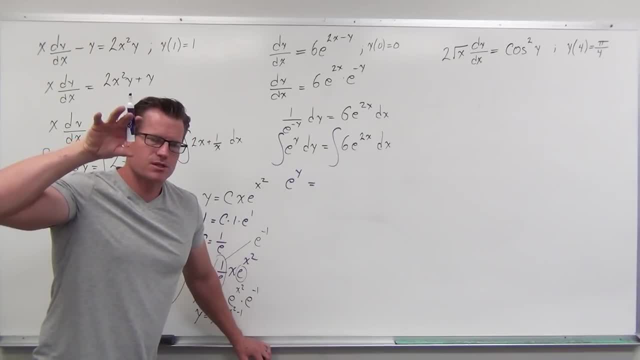 to the 2x u? u. You want to think of a? u sub here for 2x. So u equals 2x. The derivative would be 2dx, So I'm going to be dividing by 2.. One of the easiest ways that I go through it is, I think: well, what's the regular integral? 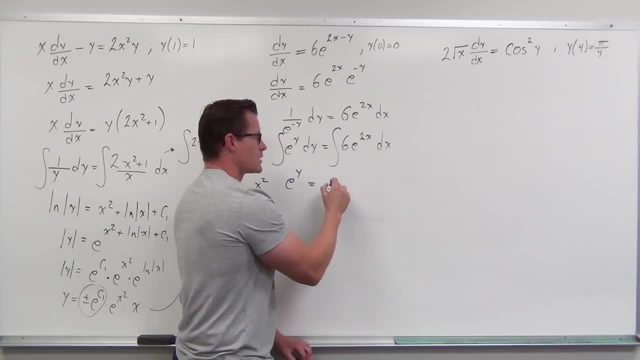 of this And I divide by the derivative of the inside. So I'll get my 6.. I'll get my e to the 2x. I'm going to divide by the derivative of that because that's how those u subs work. 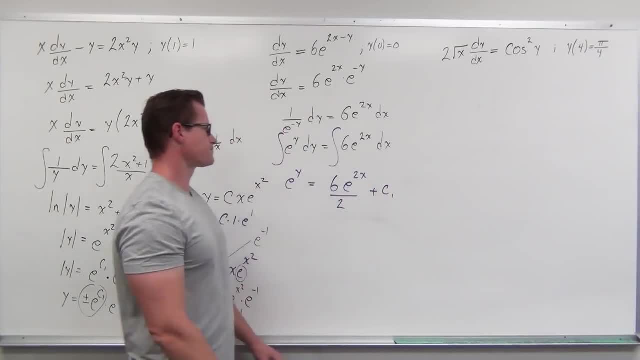 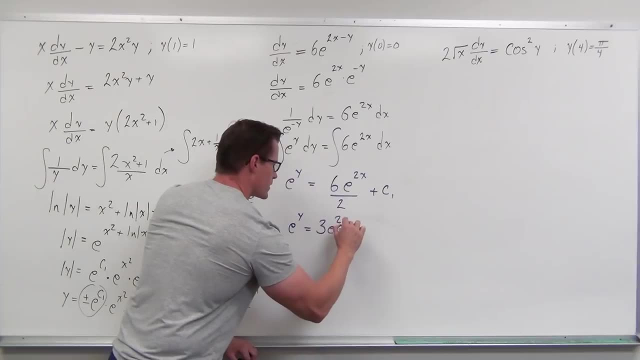 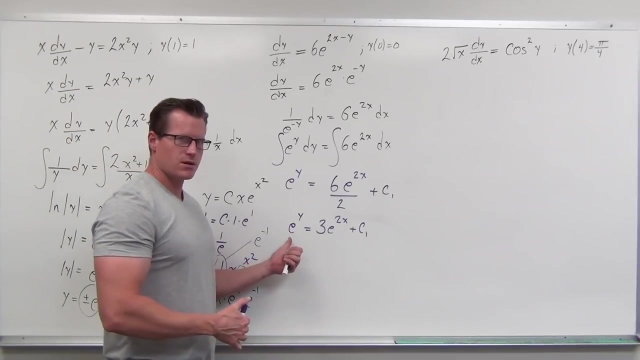 I'm going to divide by 2.. I'm going to get a plus c. So let's simplify: e to the y equals 3, e to the 2x plus c1.. Now I've already got an exponent here, So if I have an exponent here, I'm not going. 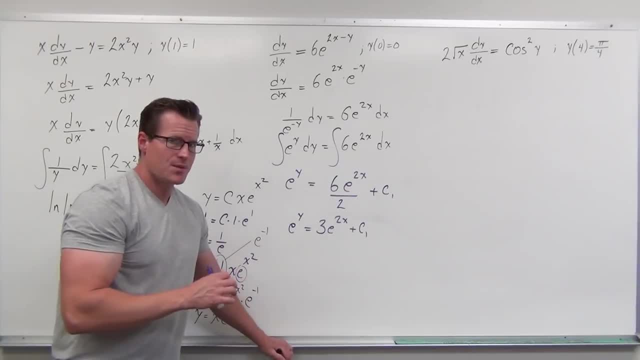 to be getting e to the c sub 1.. I'm not going to wait to plug this in. I don't have any ln's. I'm not going to be getting that plus and minus e to the c sub 1 idea. I'm going to. 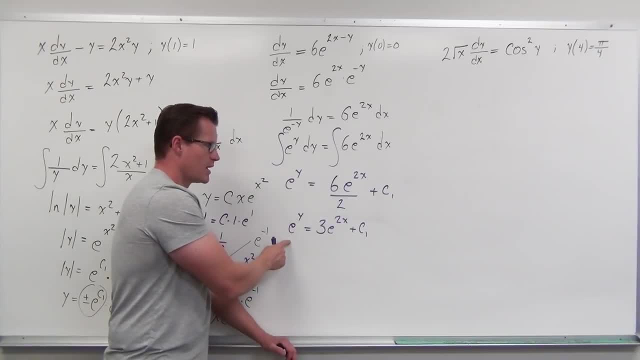 plug in my initial value now. So I have an exponential, but an exponential is not going to yield more exponentials. They would yield logarithms, which would be harder to deal with. So if you find yourself like I'm having to go backwards, 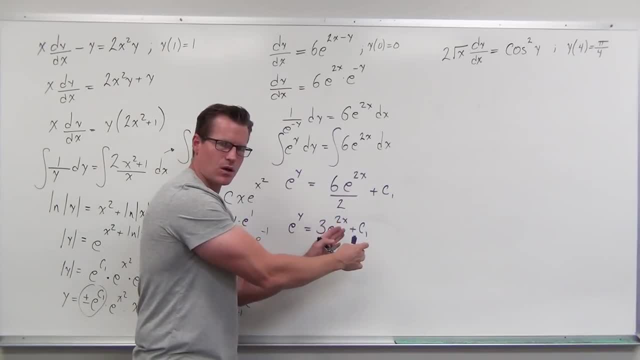 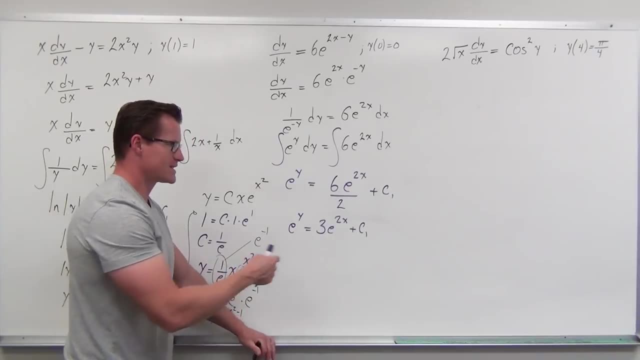 on this, y would be solved for. but if I wanted to find c, it'd be wrapped up in a logarithm. That's not great Wrapped up in an exponential. sure you can call that c, Especially if you call a logarithm c also. But it's just easier to plug it in now. So if we plug in 0 for y and 0, 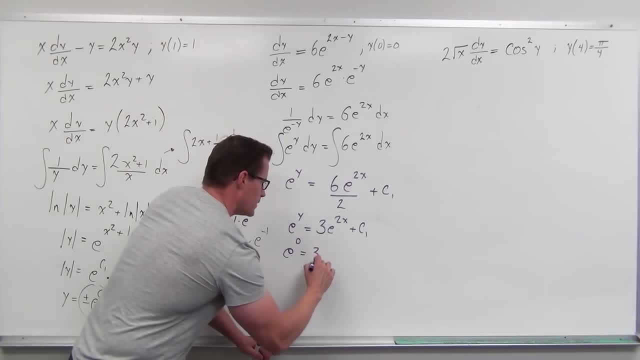 for x, we'd have e to the 0 for y 3 times e to the 0 for x, plus c sub 1.. e to the 0 is 1.. e to the 0 is 1 times 3, which means our c sub 1 equals negative 2. So subtract 3 from both sides. 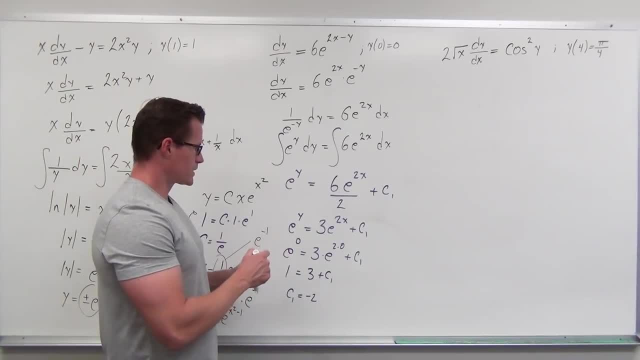 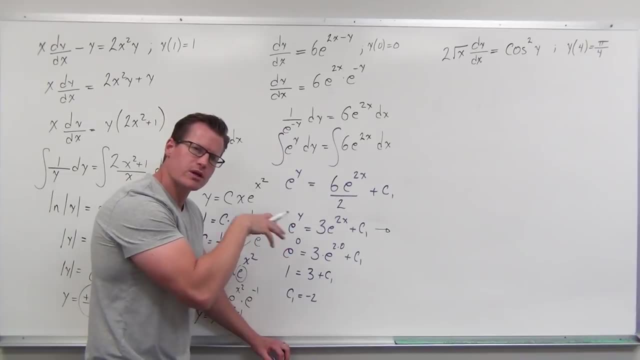 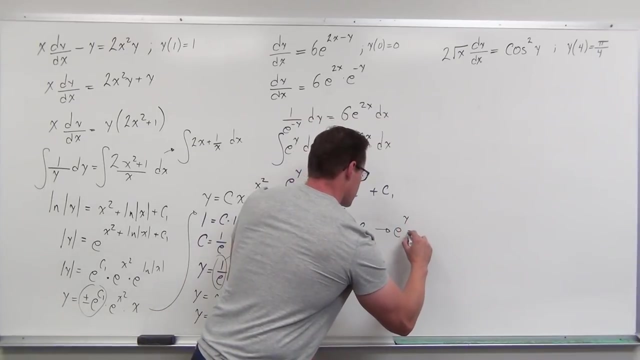 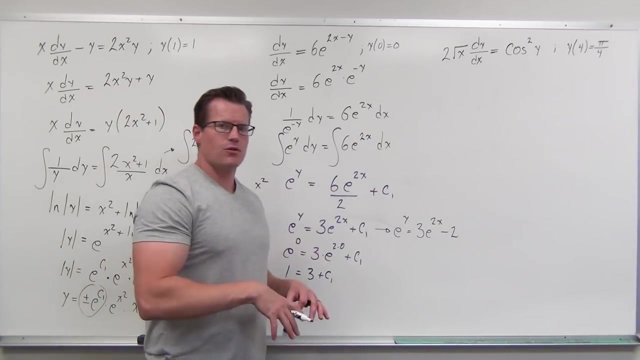 we get negative 2.. Now let's plug that back in. So we'll take our negative 2 and just change our equation from where we started, plugging our initial value to having that constant of negative 2.. So just minus 2.. Now when we solve for y, we're not going to have to backtrack to plug in for. 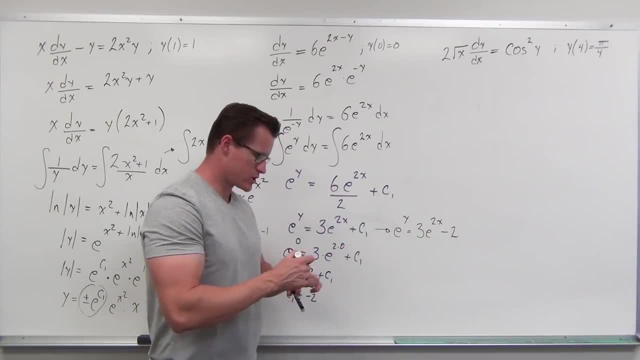 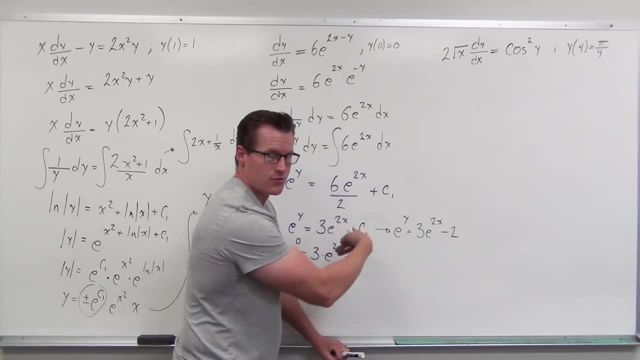 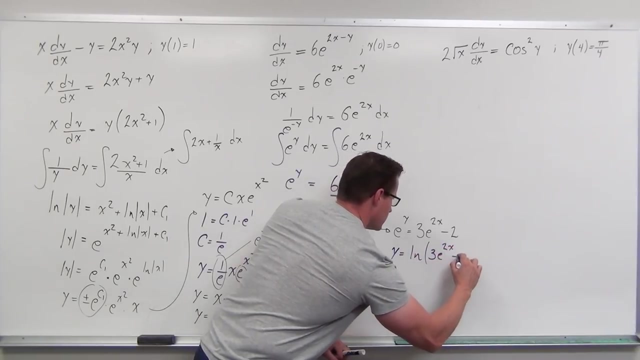 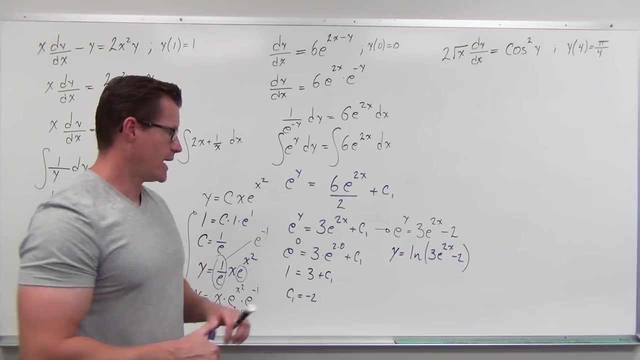 that constant. You see, if e to the y equals this expression over here, if we do ln on both sides, so e to the y equals this, then y equals ln of that Done. If you did it another way, if you had y equals all this stuff plus c1, you'd have to start undoing. 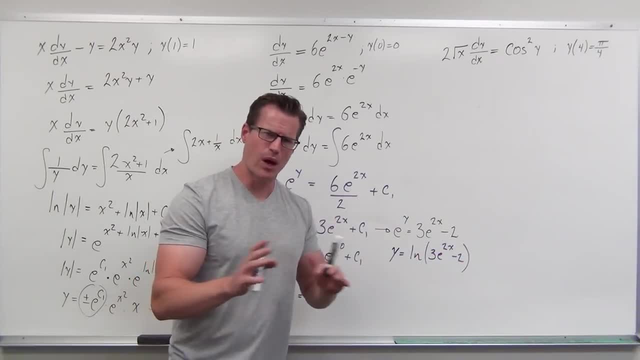 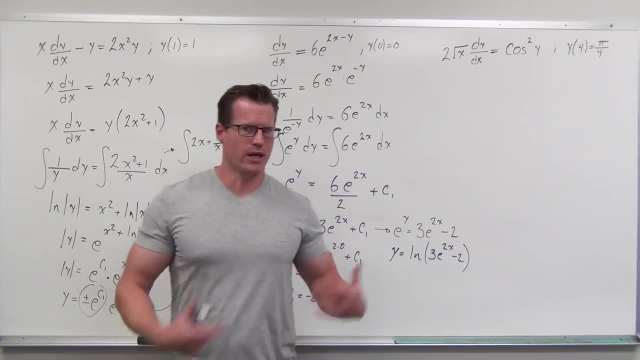 the logarithm to be able to figure out what that c would actually be. Now I want to avoid that for you. That leads to a lot of mistakes, makes it harder, makes students go. what? I don't understand any of this. Why sometimes? Why not others, If you know that you're going to be getting? 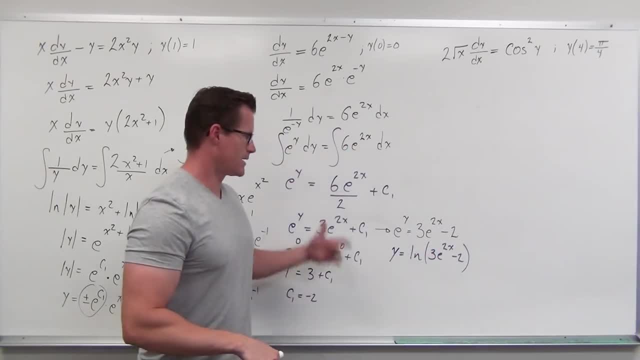 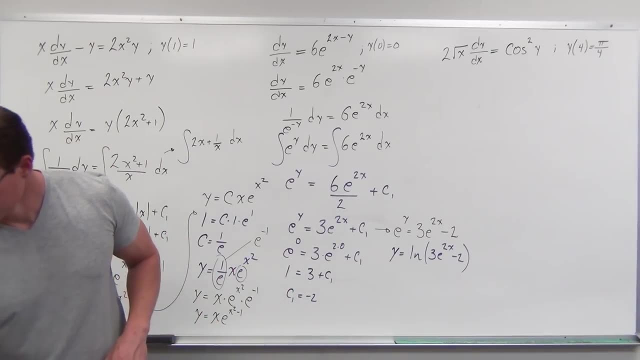 e to something with that c1,. wait, If you're not, it's best to plug it in as soon as possible. It's the idea- Okay, last one- that we got. That one's set up pretty straightforward, So we have. 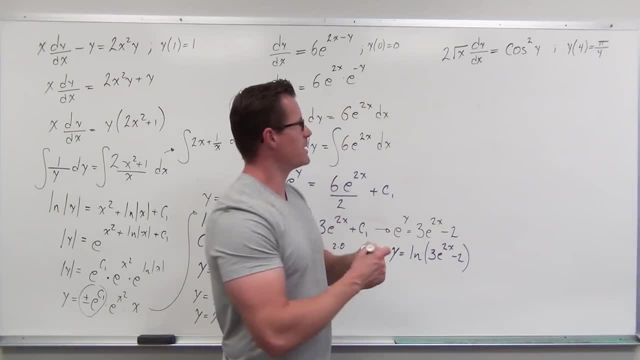 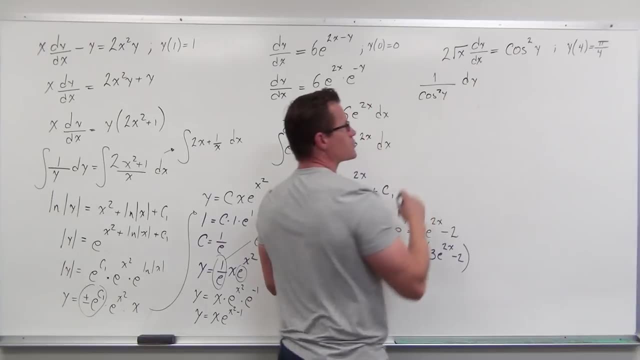 some x's here, we get some y's here. We're going to switch them. We're going to make sure that we set this up as function of y dy, So function of x dy equals function of x dx. Then we integrate. 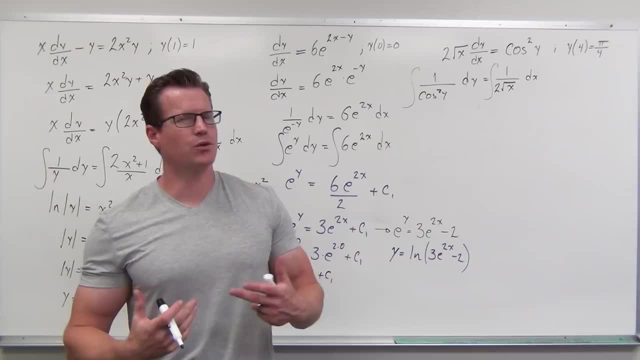 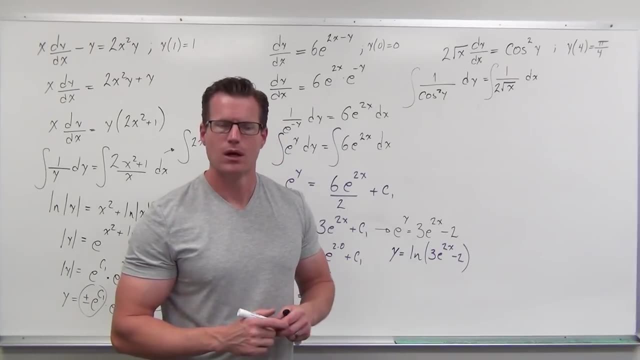 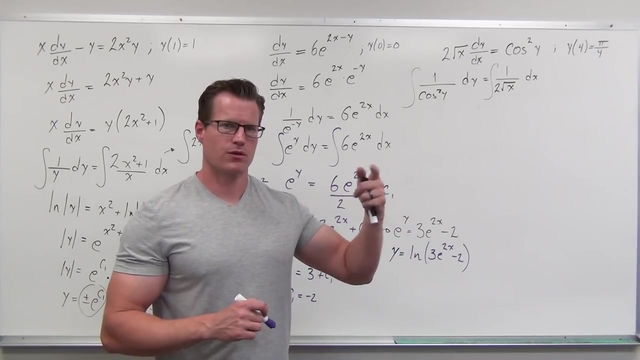 Now, when stuff doesn't look familiar to you or look good, change it. So 1 over cosine, squared y doesn't look that great, You go, that's not on my table. Well, yeah, of course it's not on your table, Because if secant is 1 over cosine, 1 over cosine gives you secant, And if 1 over cosine, 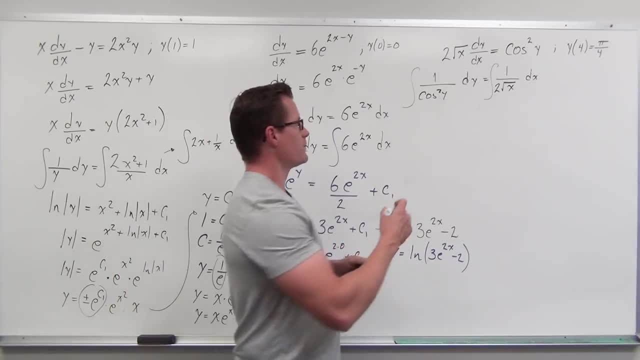 squared is what you have. then you have 1 over cosine squared. So you have 1 over cosine squared. Then you're going to have secant squared. So on the left-hand side we have an integral of secant squared. y dy, It's actually really nice On the right-hand side. 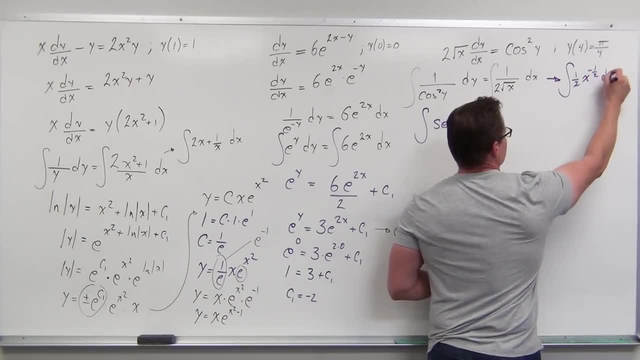 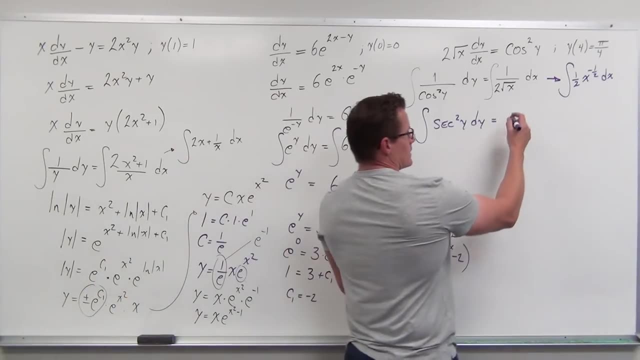 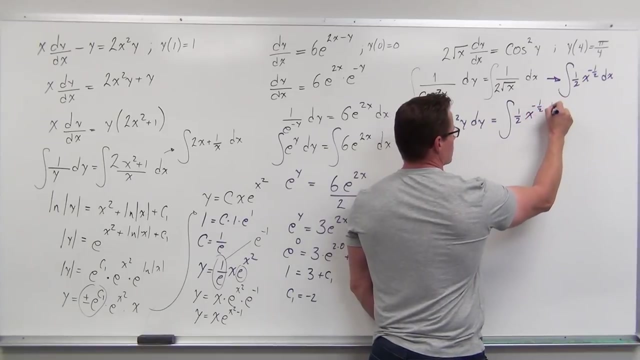 we've got an integral of 1 half x to the negative 1 half which we had in the previous video. Well, that is going to give us 1 over cosine squared y dy. On the right-hand side, we keep our 1 half. We always add to our exponent, So that's 1 half over. 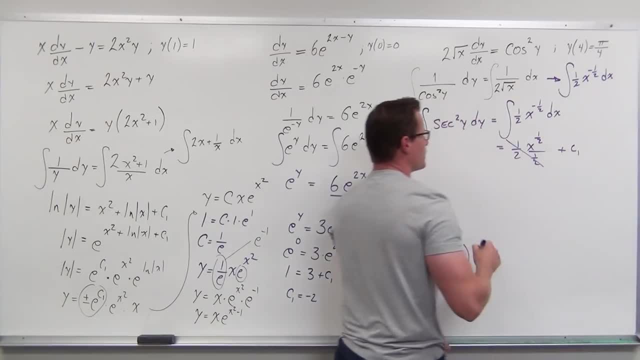 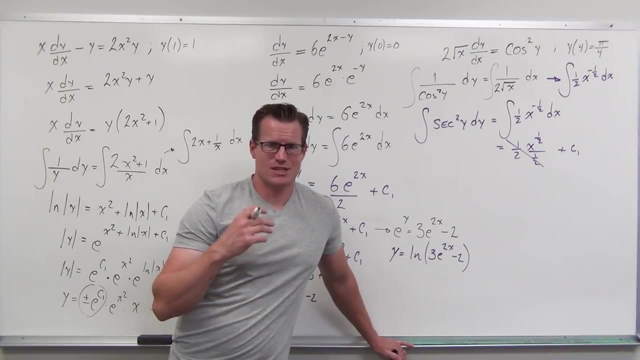 1 half, And our 1 halves are gone, Plus c sub 1.. On the left-hand side: well, this is kind of nice. The integral of secant squared y dy is just tangent y. The derivative of tangent y gives. 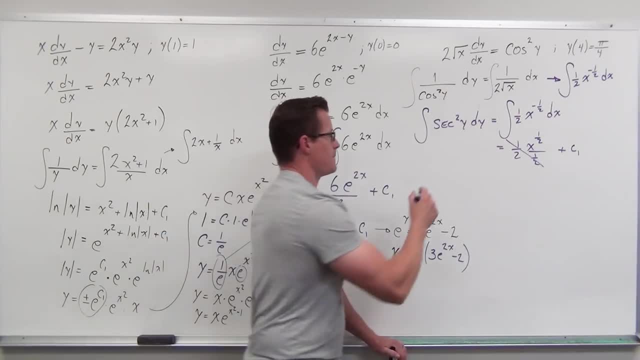 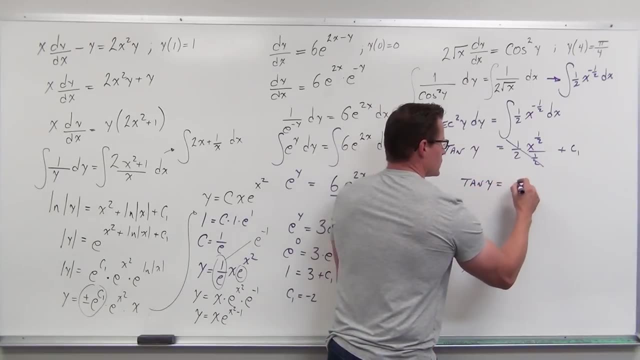 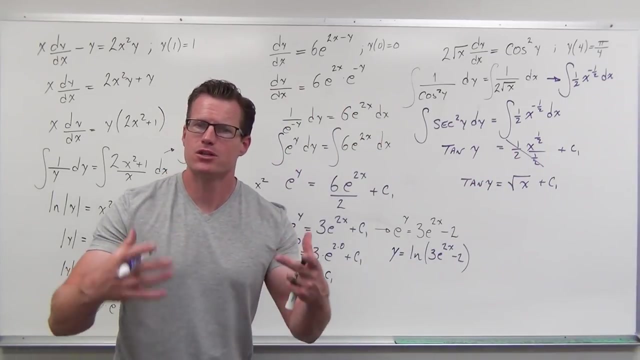 you secant squared. So the integral of secant squared gives us tangent y. So we know that tangent y equals square root of x plus c sub 1.. x to the 1 half, It's all we've got. That's the square root of x plus c 1. Now think in your head: Is this going to give you any? 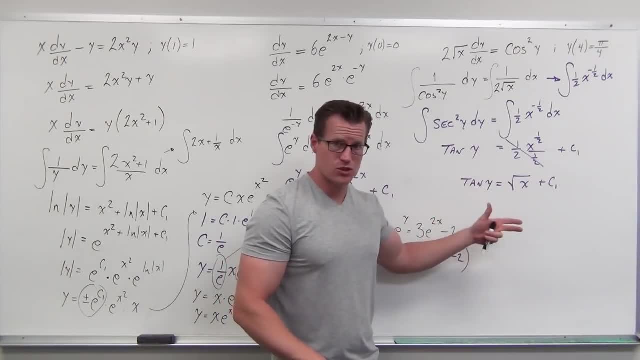 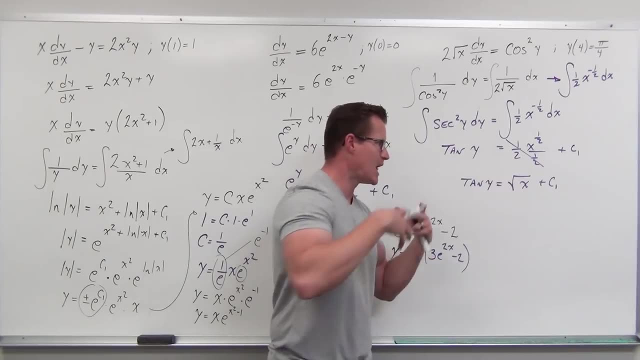 exponents e to the c 1, stuff like that. If the answer's no, then plug in your initial value. now, If the answer's yes, then you wait until you wrap it up in that larger arbitrary constant, Then you plug in your initial value. So right now I know that y of 4 equals pi over 4.. That means 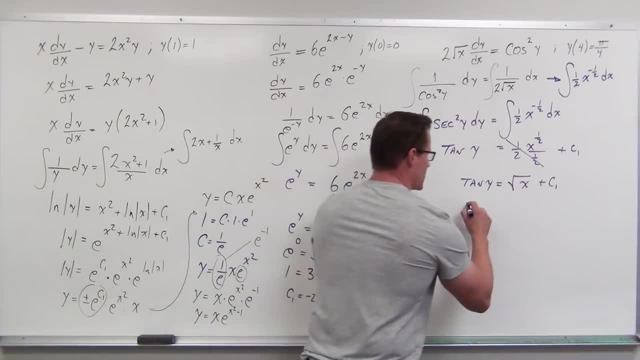 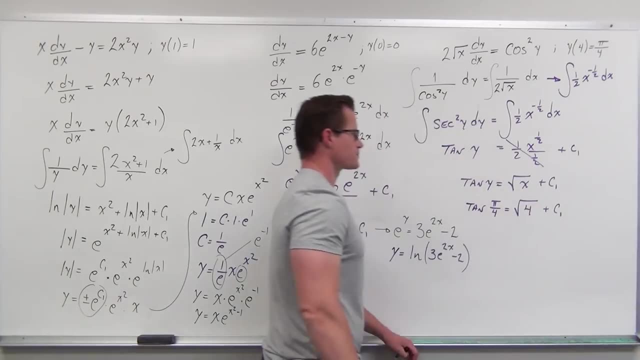 that y is pi over 4 when x is 4.. So tangent pi over 4 equals square root of 4 plus c sub 1.. y becomes pi over 4.. x becomes 4.. And this is really nice, because tangent of pi over 4 is 1.. 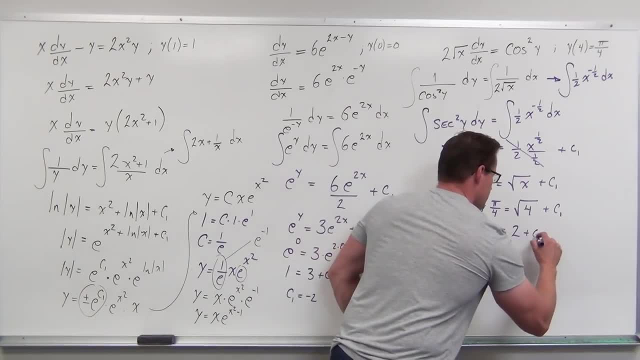 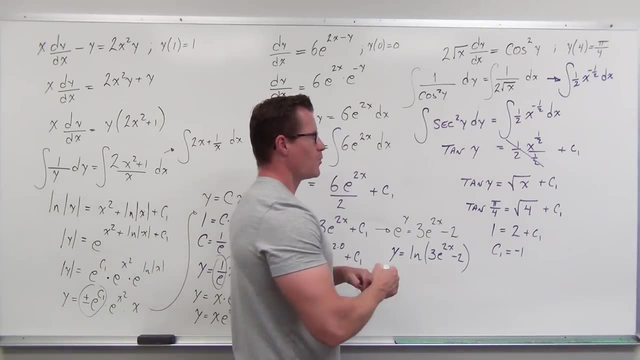 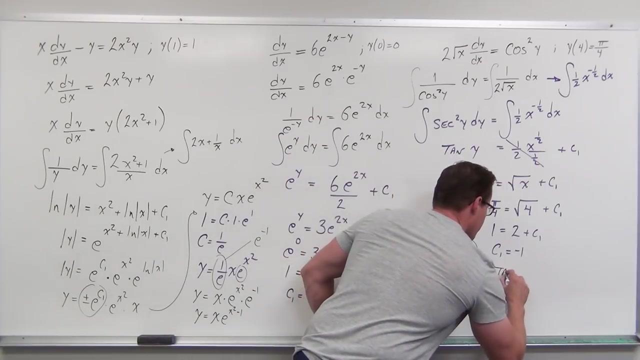 We got that. Square root of 4 is 2 plus c sub 1.. That says c sub 1 equals negative 1.. Let's just plug that back in. So from where we started plugging in our initial value, from right here we have tangent of y equals the square root of x. 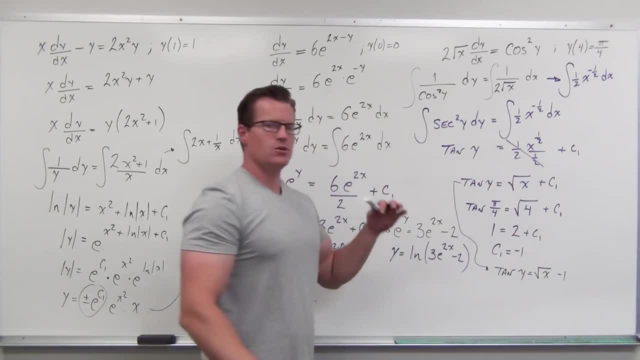 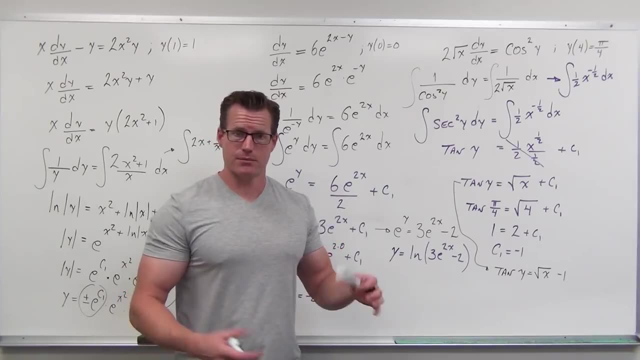 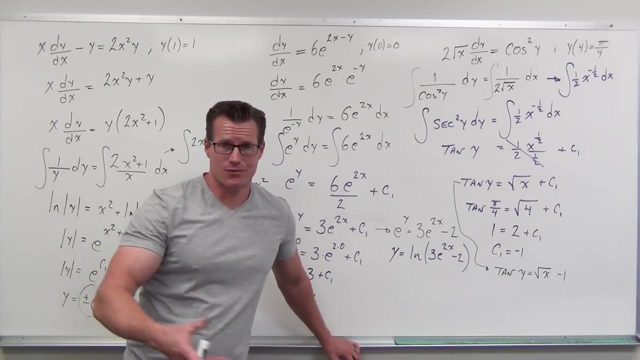 minus 1.. If you didn't plug in the initial value now and you solved for y, you'd have to be going backwards a lot to figure out what that constant is. Now, if we have tangent of y equals our expression, we know. if tangent of y equals an expression, y equals tan inverse of that expression. 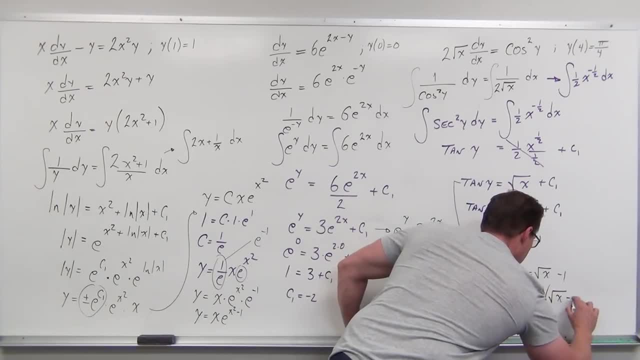 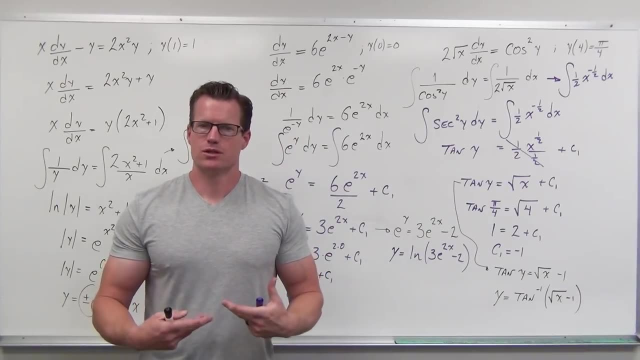 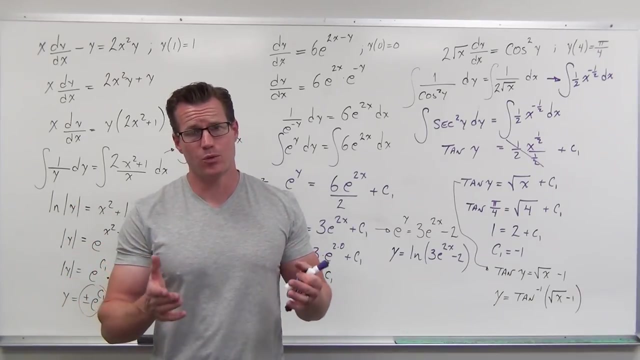 That's a particular solution to that differential equation that goes through that point. That's what we're looking at doing with initial value, So not much of a difference besides understanding when to plug in that initial value. That hopefully, will help you a lot, because that's rarely explained. 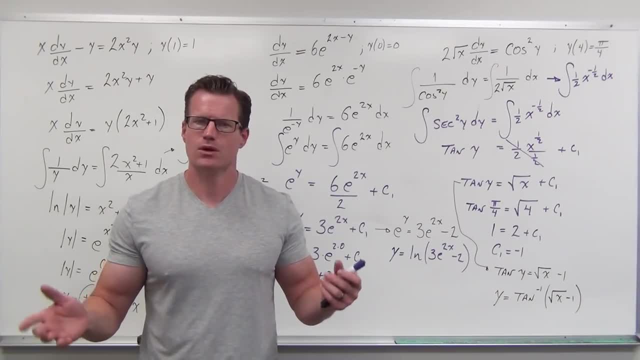 Like: when do you plug it in soon? When do you plug it in later? Do you plug it in the same place every time? No, you don't. Well, at least not according to me. Textbooks don't really explain that. Some teachers don't explain that very well, Like.